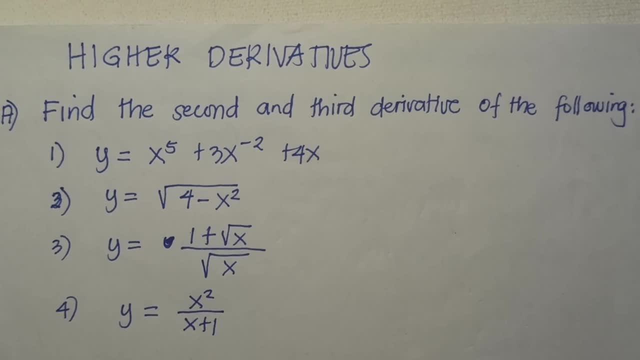 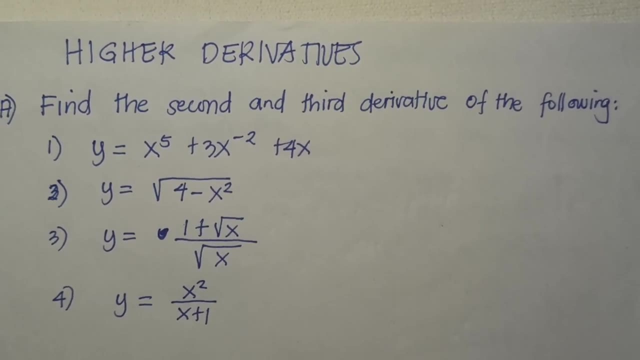 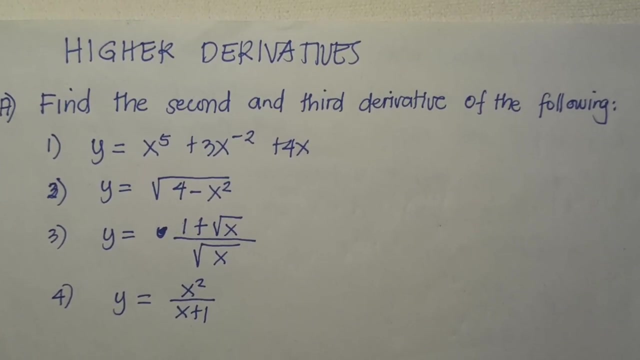 derivative And we need to find the third derivative. just take the derivative of the second derivative in order for you to get the third derivative of the function. So we have here the problem. y is equal to x raised to 5 plus 3x, raised to negative, 2 plus 4x. Number two, y, is: 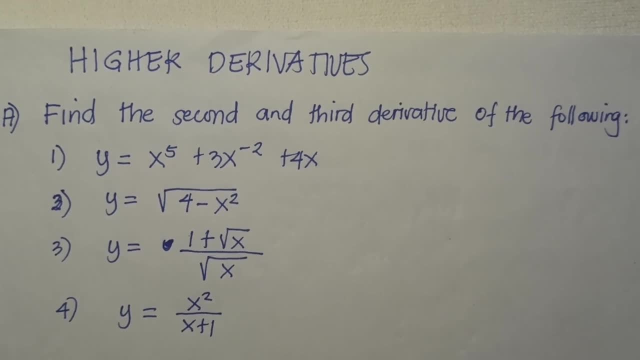 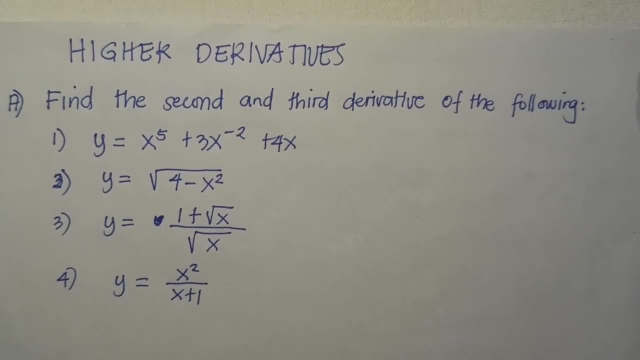 equal to the square root of 4 minus x squared. And number three, y, is equal to 1 plus the square root of x over square root of x. And four, y is equal to x squared over x plus 1.. So get ready. 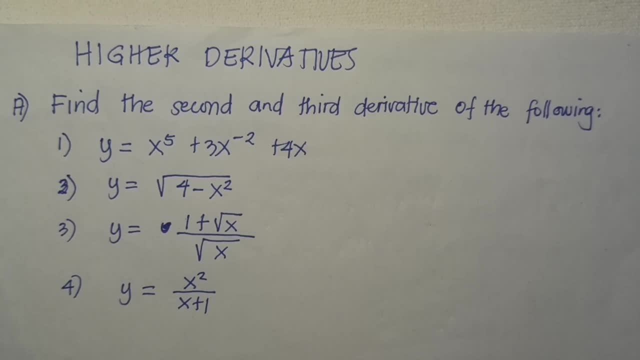 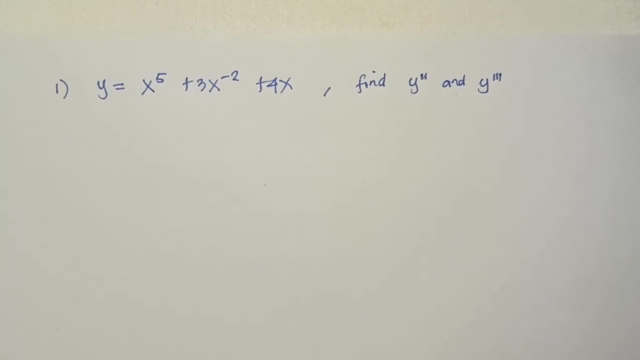 because we will be solving number one for this item. Okay, so let's proceed with number one. So y is equal to x raised to 5 plus 3x, raised to negative 2 plus 4x, And we need to find the second. 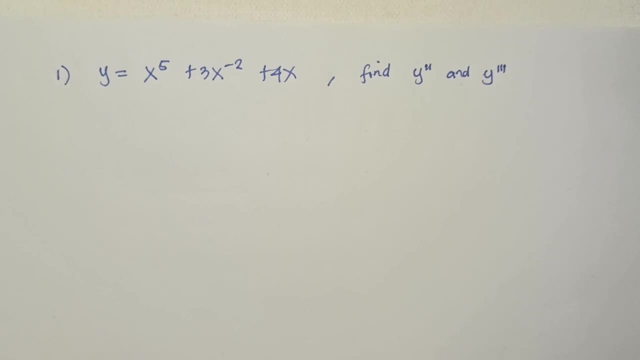 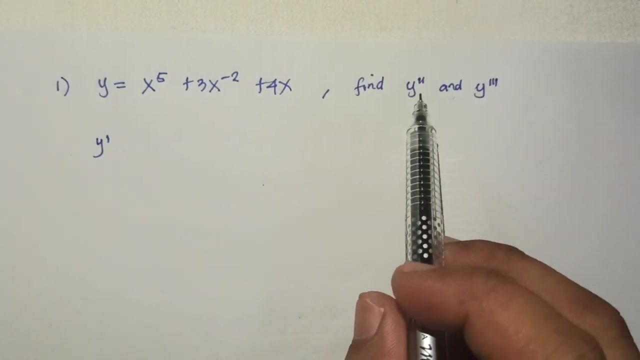 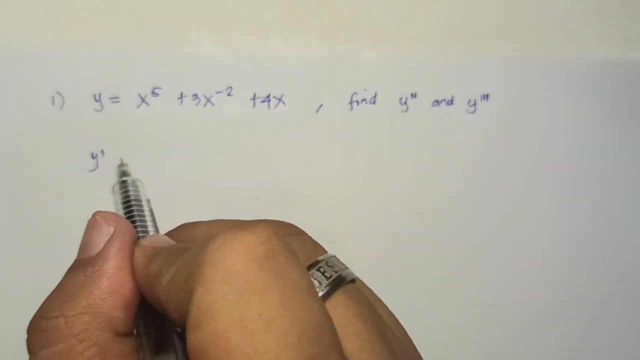 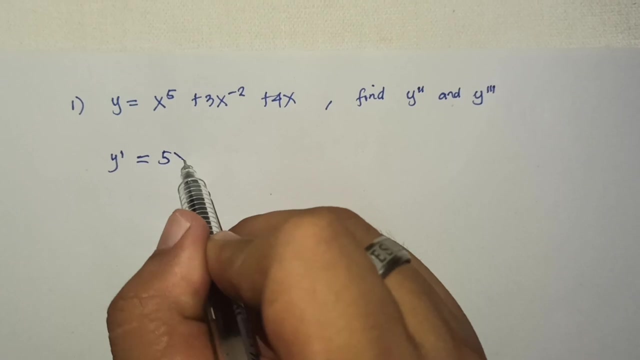 derivative and the third derivative. So this is the basic one. So y prime: first we need to find the y prime in order for us to get y double prime and y cube or y triple prime rather. So y prime is equal to. so we have to differentiate this one. So bring down this 5, then subtract it by 1.. 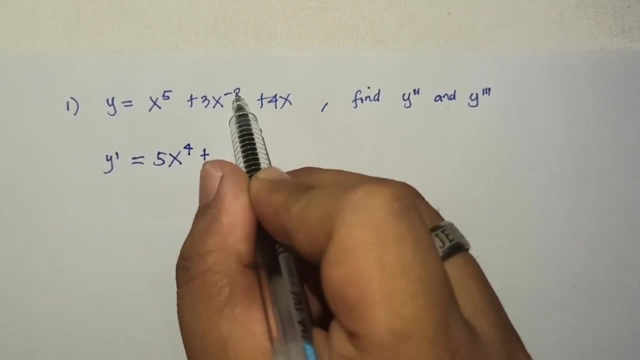 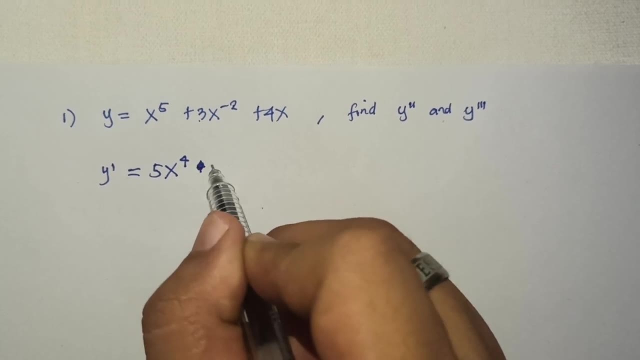 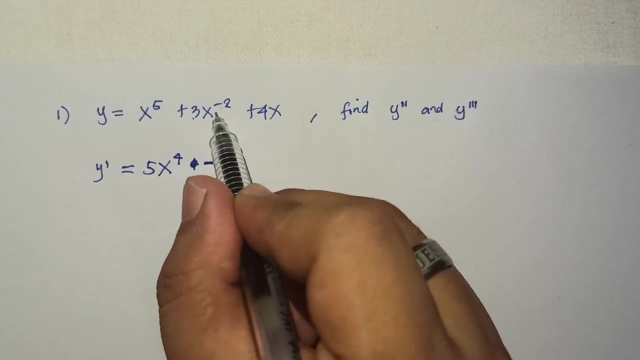 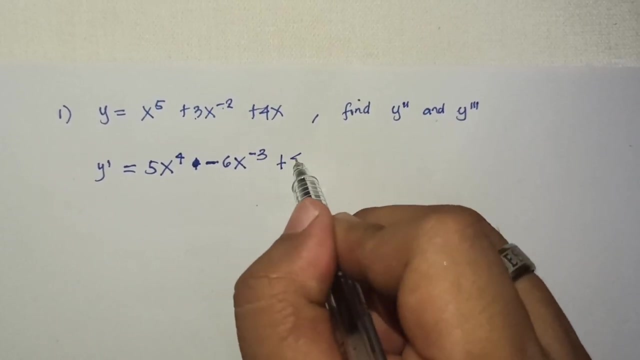 So the result is 4 plus negative 2.. 2 times 3,, that is negative 6.. So we have to change parts. So this is minus 6x. subtract it by negative 1, that is negative 3. Then plus derivative of 4x is equal to 4, of course. 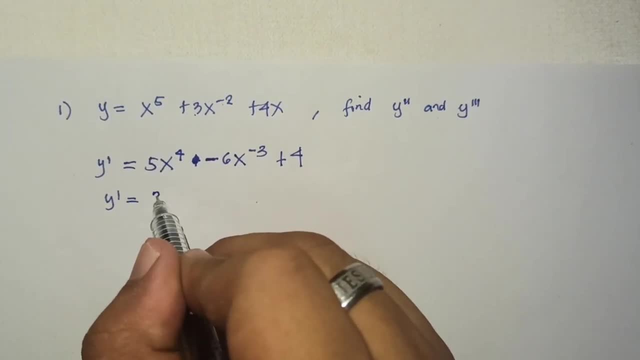 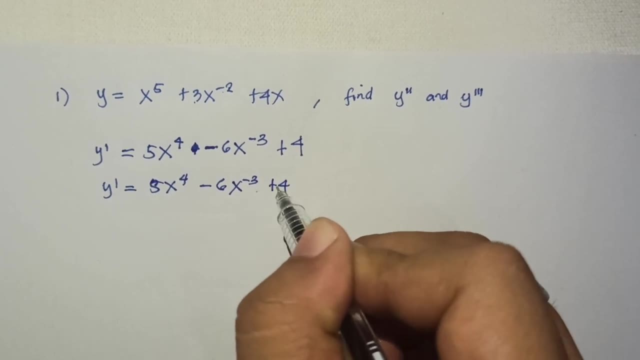 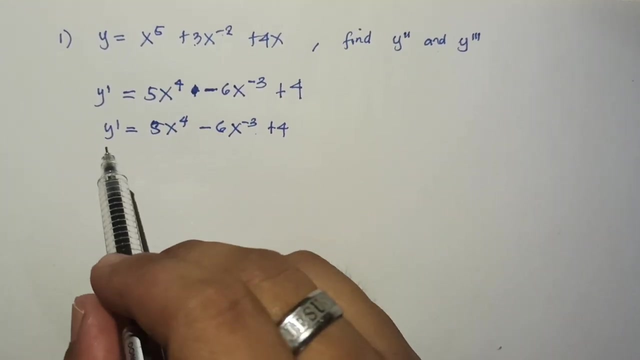 So y prime is equal to 5x raised to 4 minus 6x, x raised to negative, 3 plus 4.. So this is the first derivative. In order for you to get the second derivative, we need to take the derivative of the first derivative. So therefore, for the 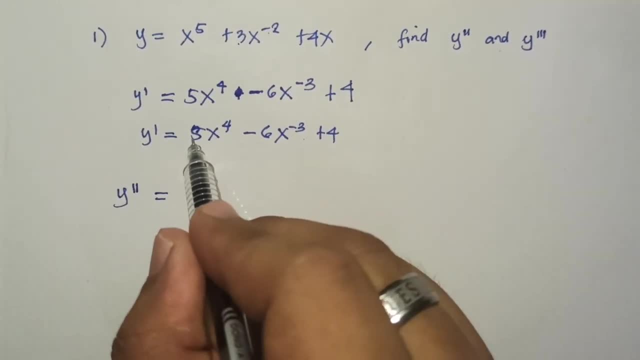 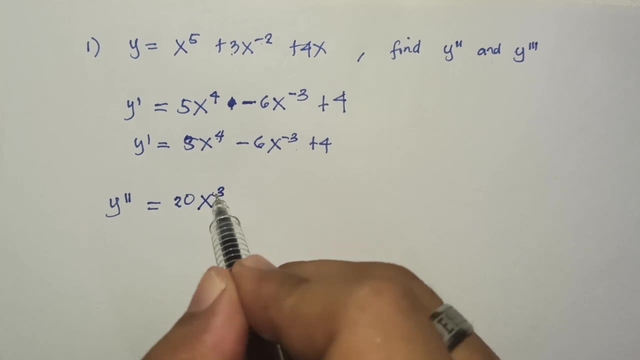 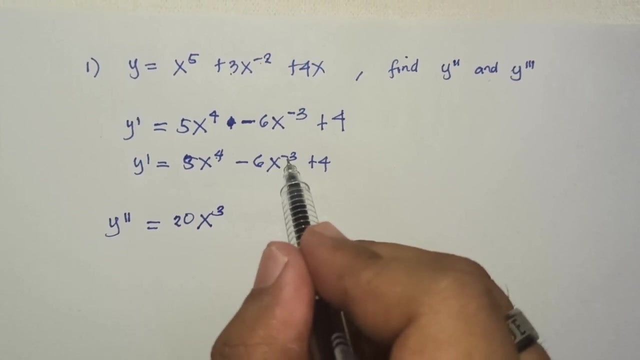 second derivative: we have multiply this part, So this is 20.. So 4 times 5, that is 20x, 4 minus 1, that is 3.. Then negative 3 minus 6, that is negative. 3 times negative 6, that is 18 plus 18.. x raised to negative 3 minus 1,, that is negative 4.. 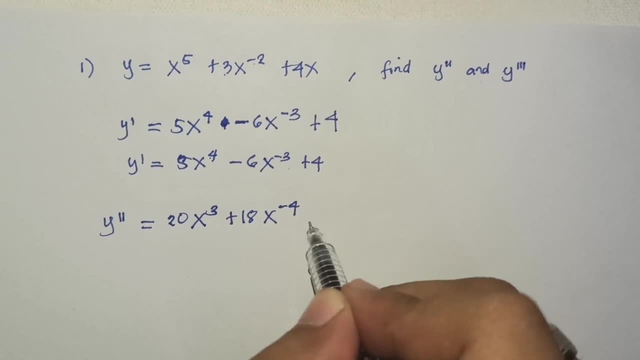 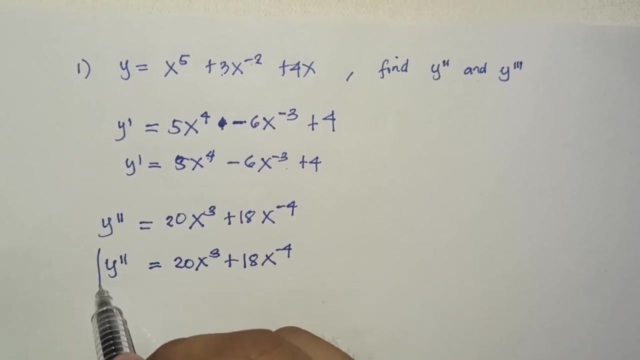 And derivative of a constant is equal to 0. So therefore we will not write it here anymore. So y double prime. So the resulting of this one is 20x cubed plus 18x raised to negative 4.. So this is. 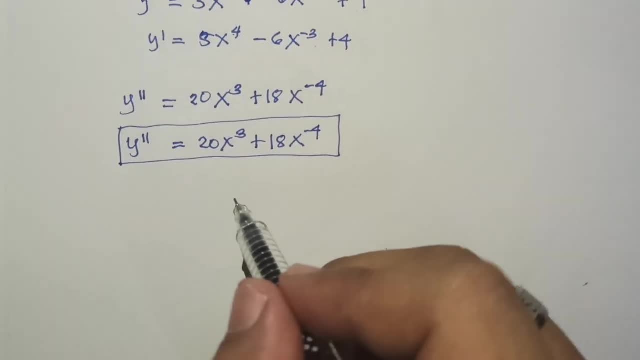 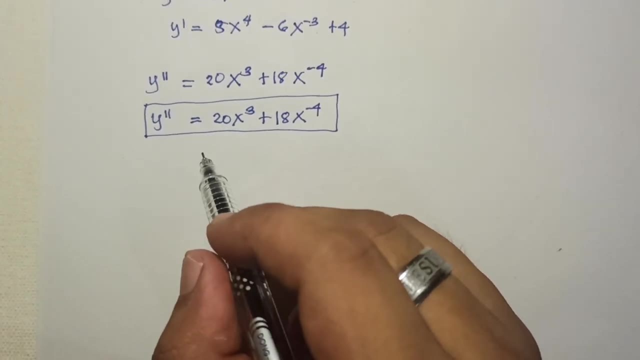 our derivative. So that means we will add up the derivative which is 43 upon 10, plus 500 to darius. Then we subtract the 2,, that is 90. Since you have the derivative of the 1st derivative and the 2nd derivative, that is the derivative which is the 2, that is negative 2.. 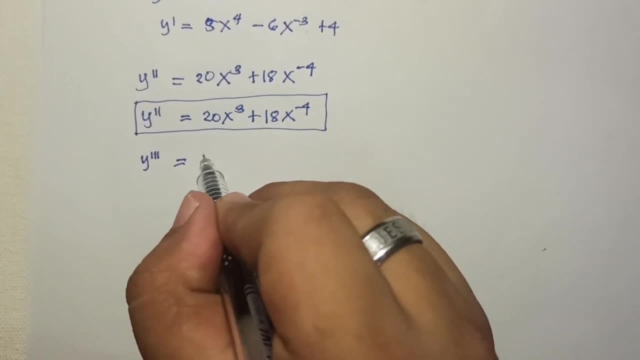 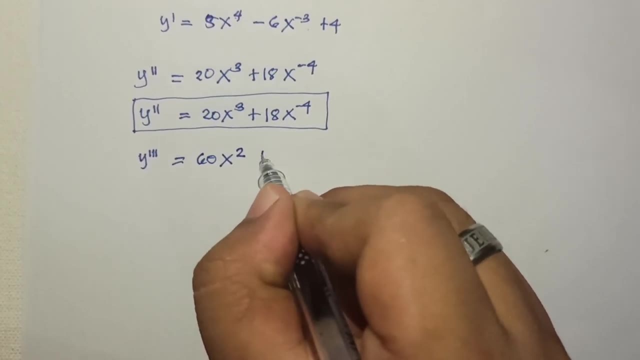 So we ask for the second derivative in order to get the 2nd derivative. So, taking for the 3rd derivative, take the derivative of the second derivative in order for you to get the 3rd derivative. So y third derivative is equal to –ہ, this is 60x, and this is 3 – 1, that is 2.. And this is – danced, This is – derivative of. the help of our second derivative. So massage between her with the help of Еще, to the help of my ideas, was to say, when we get stable, Then we have to mortgage the verb. So 3 minus 4, that is 16x squared 1 of the way in hand. 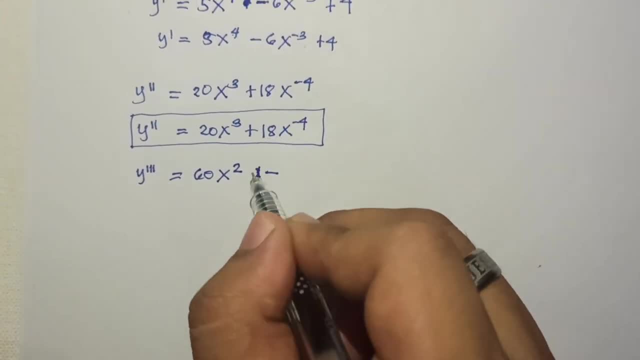 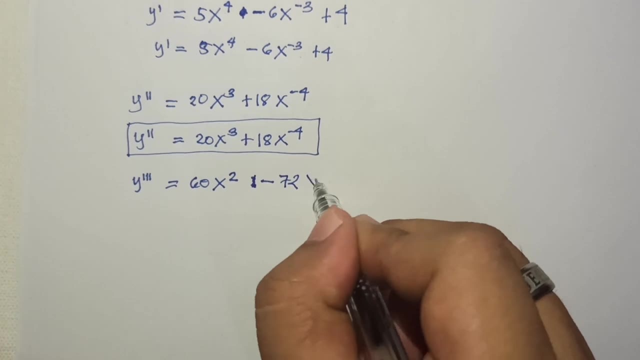 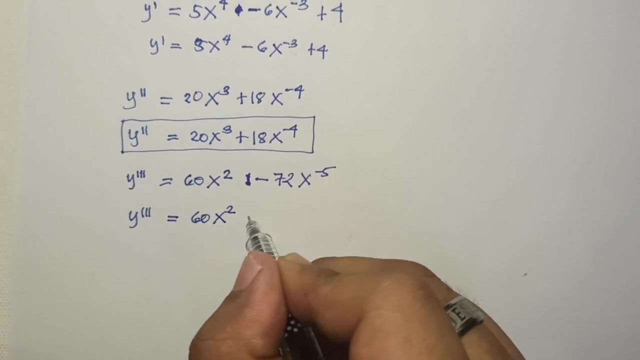 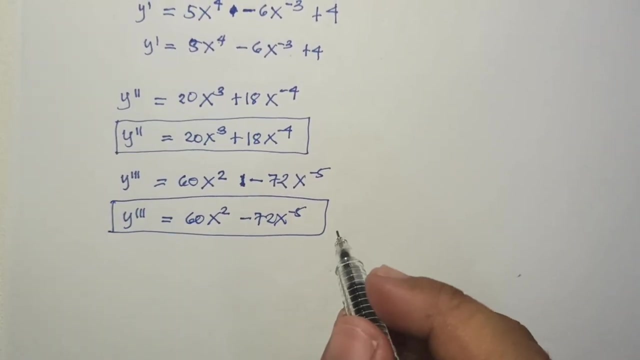 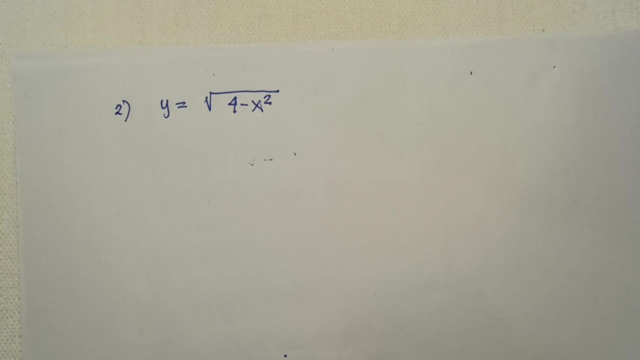 this is minus. so negative 4 times 18, that is 72. then x raised to negative 4 minus 1, that is x raised to negative 5. therefore the third derivative is equal to 60 x squared minus 72 x raised to negative 5. so this is question number one. okay, so let's proceed with question number two in this. 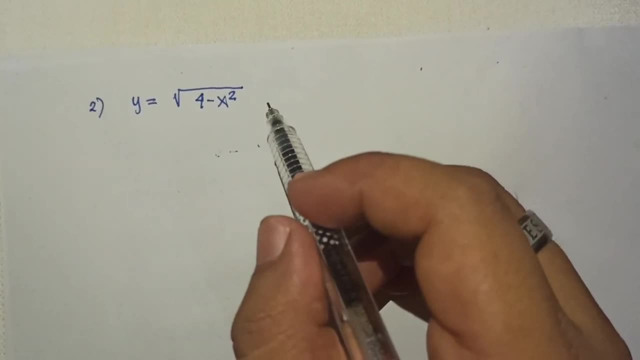 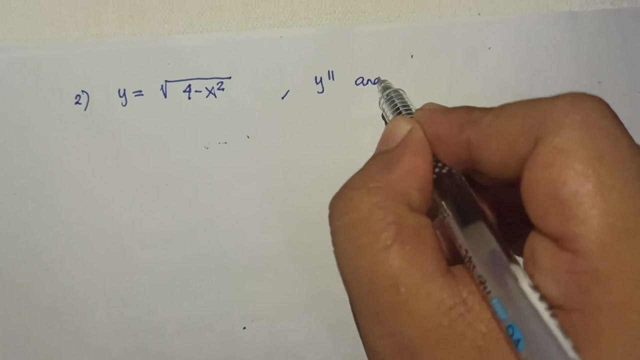 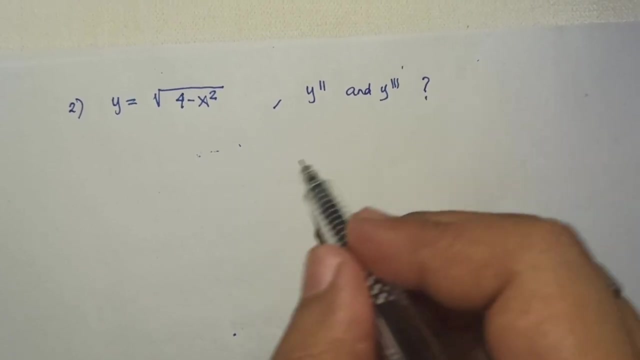 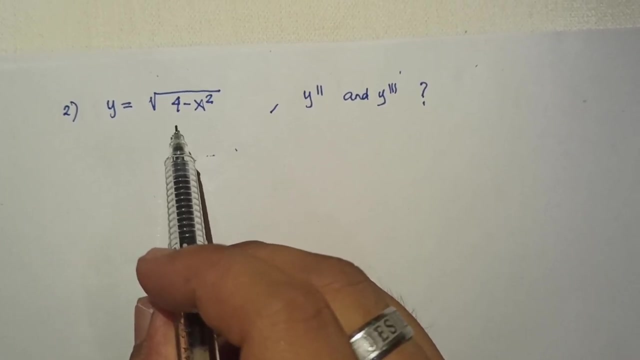 case we need to find, for: y is equal to 4 minus x squared square root. so we need to find again double prime and triple prime or the third derivative. so this is our question, okay, okay. so in finding this one first, we need to express this one into exponential form. so y is equal for. 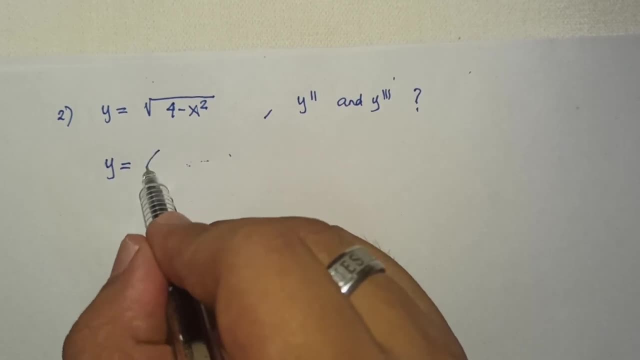 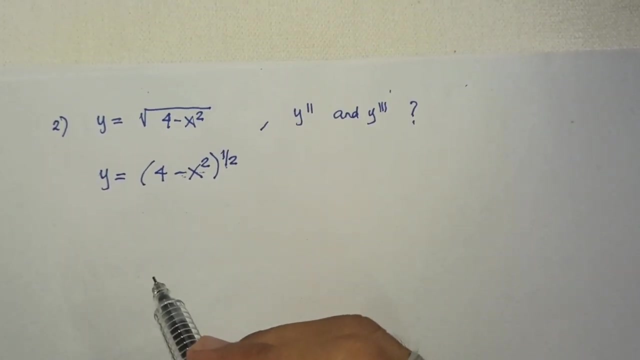 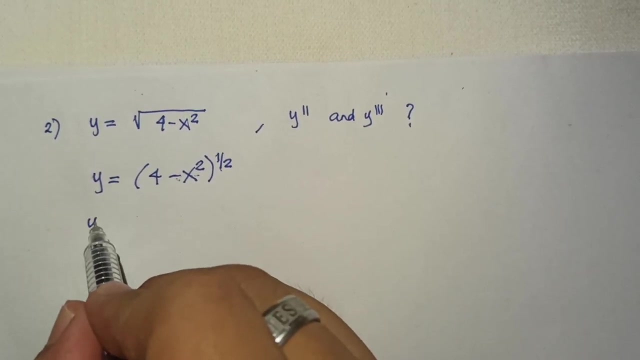 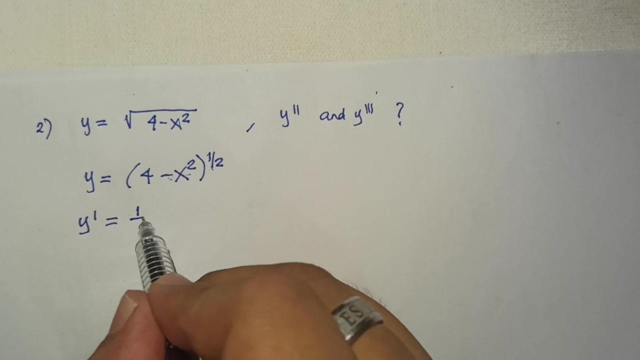 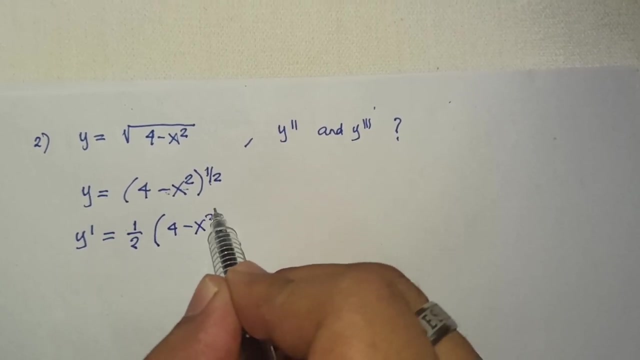 us to have an easy way of solving. so 4 is easy when it is exponential. so we have one half. so 4 minus x squared raised to one half. so in this case we need to take the derivative of this part. so, following the chain rule, the chain rule, so we have to have one half. so chain rule, so 4 minus x squared raised to one half. 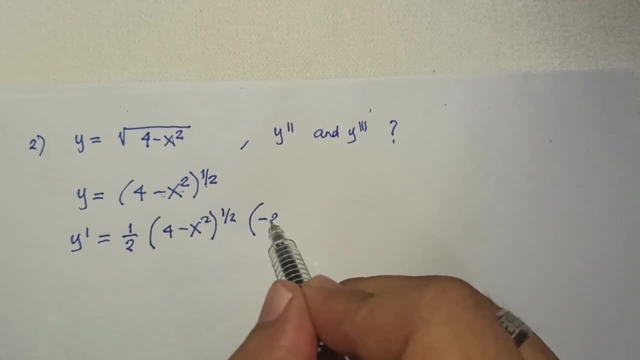 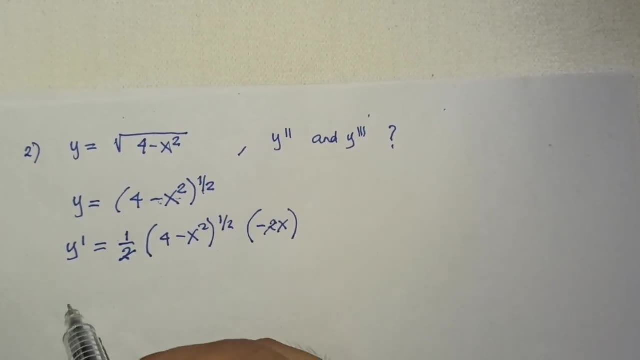 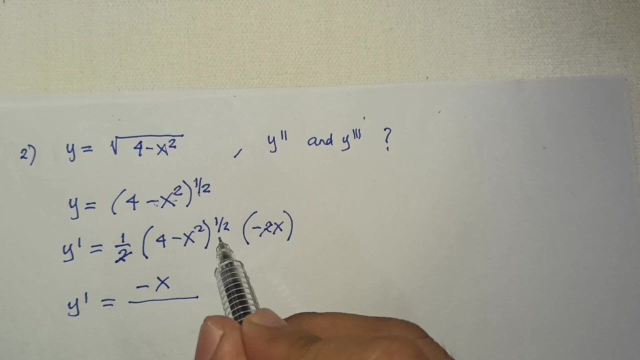 times the derivative of this one is negative 2x, so first we need to cancel this part. so we have y prime is equal to negative x and this is the derivative of this one. so we need to cancel this derivative of this one. so this is the derivative of this one. so this is minus 1 rather, so this this. 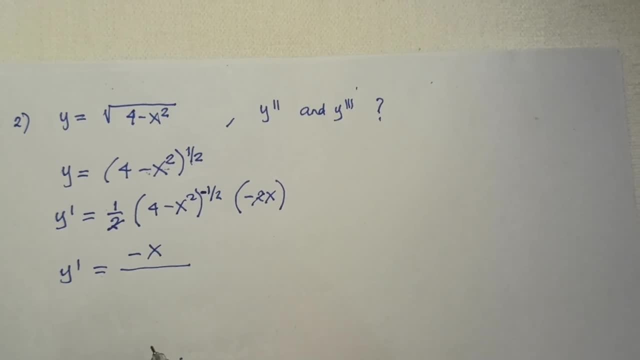 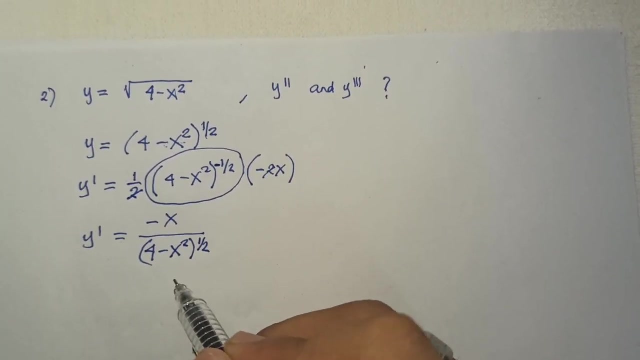 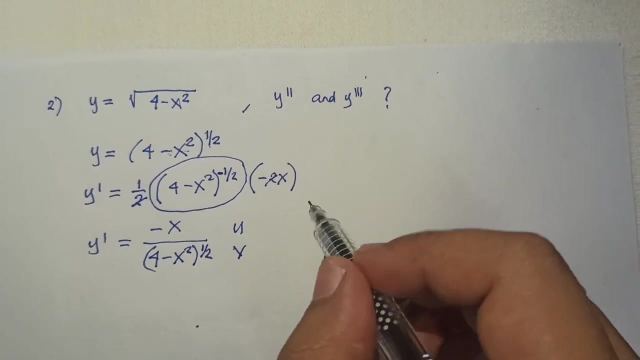 will become negative 1 half, because one half minus 1, that is negative one half. so therefore this part will be at the denominator so forth in order to have a positive sign. so this is one half. so this is in the form of u and v to take for the second derivative. so the second. 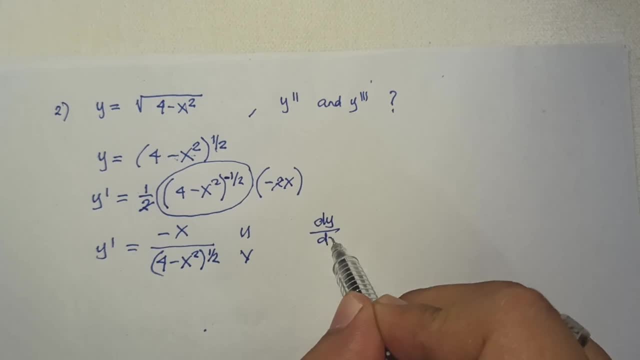 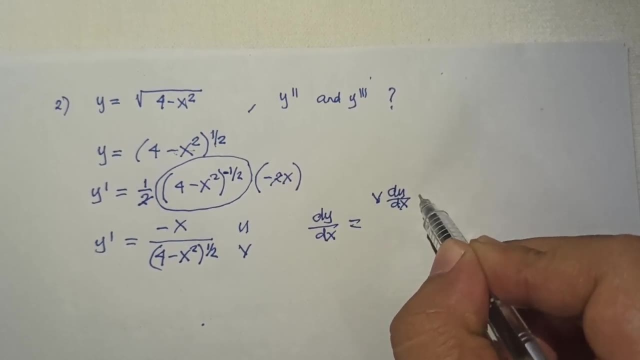 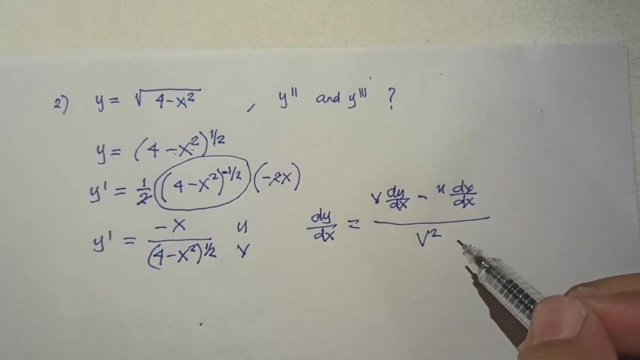 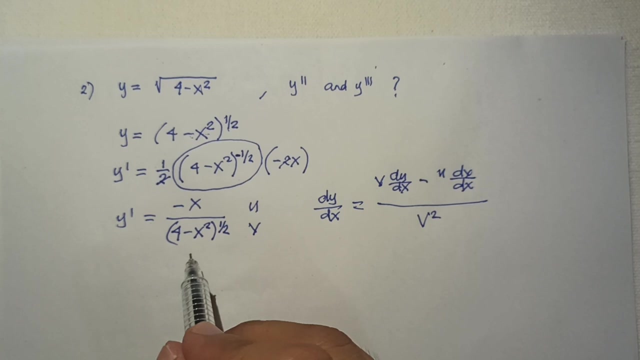 derivative is equal to dy over dx, is equal to v du over dx, minus u dv over dx over v square. So this is the formula in finding quotient rule. So in quotient rule, so we need to apply for this one to get for the second derivative. So y double prime is equal. 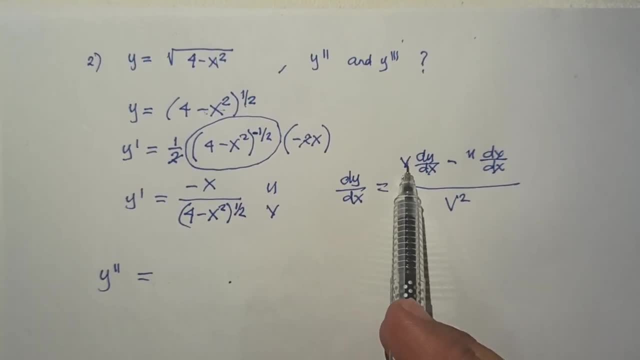 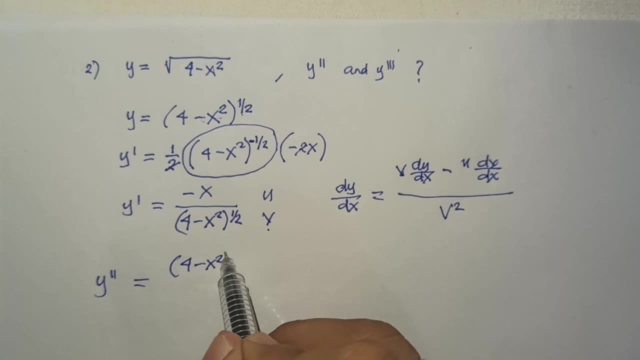 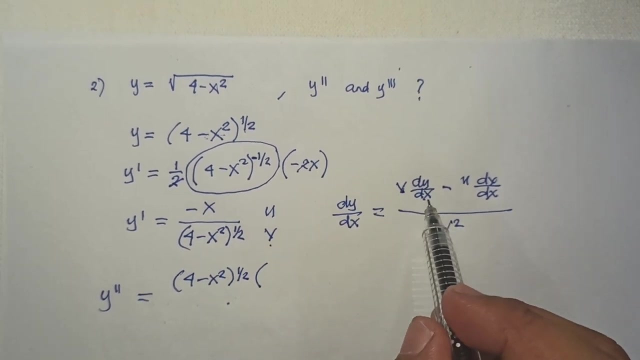 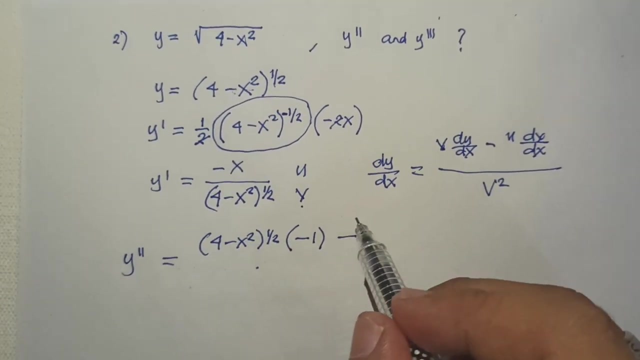 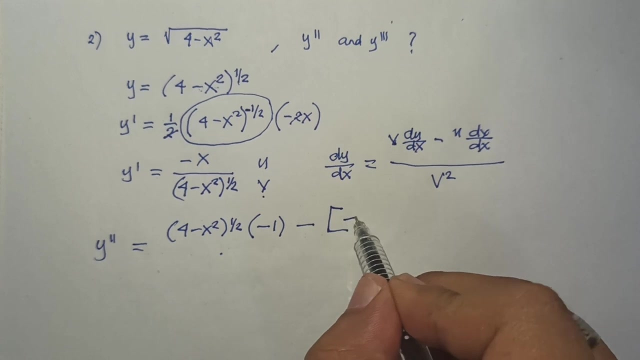 to so. first we have to copy v. So this is the v we need to copy. So we have 4 minus x, squared raised to one half times derivative of u with respect to x, which is negative 1.. Minus we have here, so we have to take this for u, copy the u, which is negative x times. 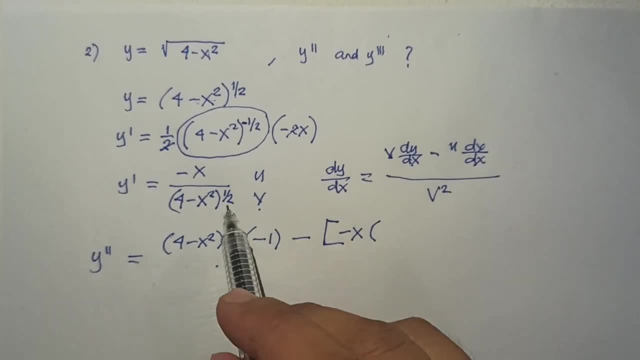 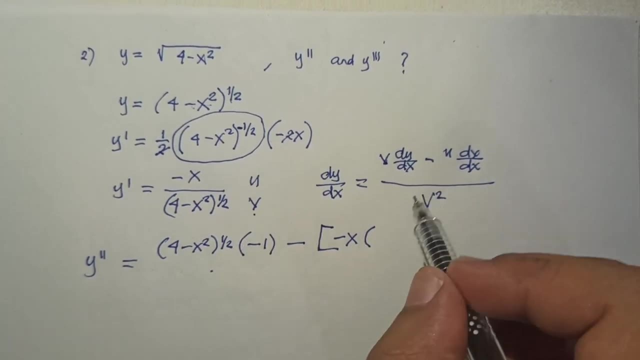 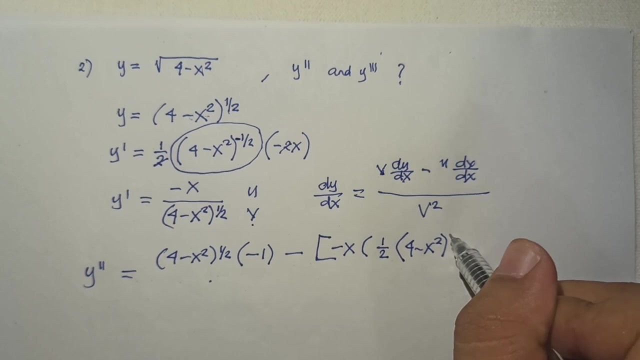 we have the derivative of v, So the derivative of v. okay, the same process with this one. This is the derivative of v here, So one half times 4 minus x squared. Next we need to simplify: y double prime is equal to negative, 1 half times negative. 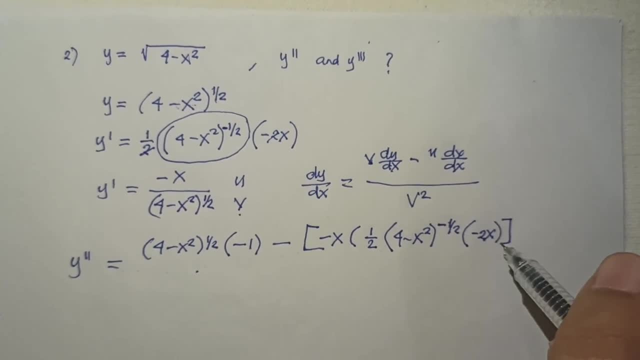 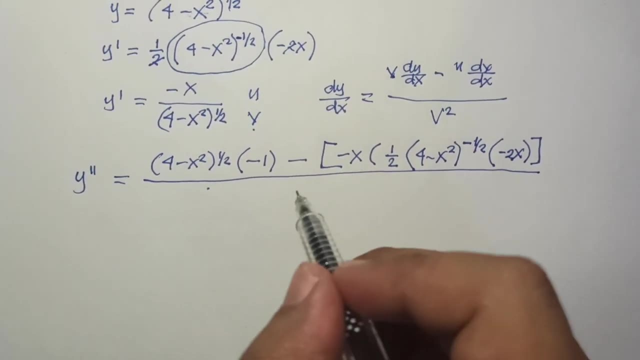 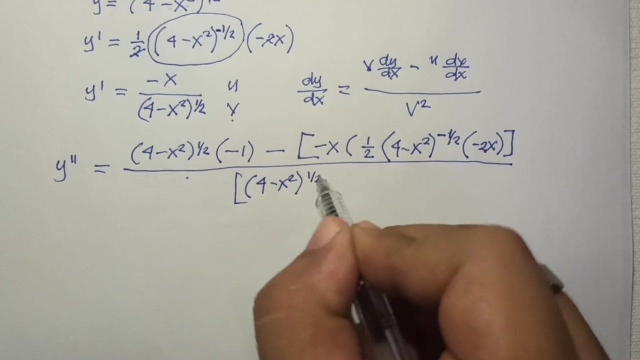 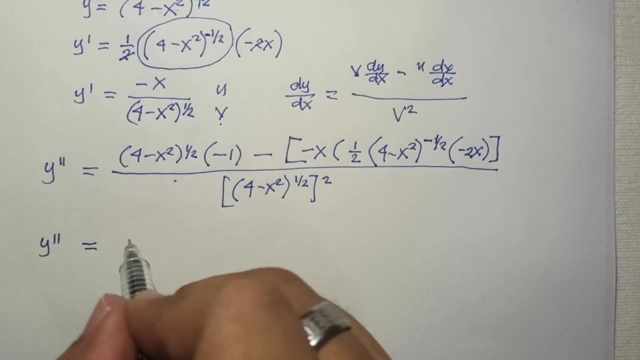 2x. Okay. so by the use of chain rule over v square, So v here is: 4 minus x, squared raised to one half, then square. Next we need to simplify y. double prime is equal to negative 1 half times negative 2x. Okay. so by the use of chain rule over v squared, So v here is: 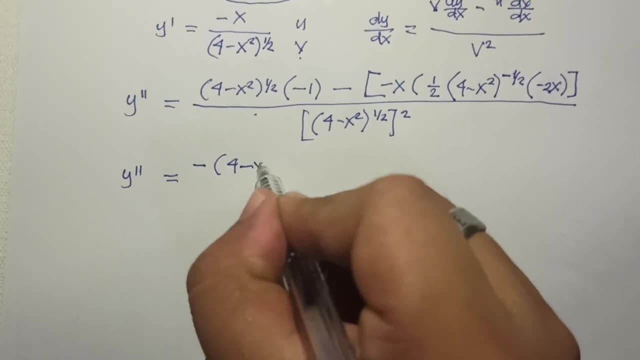 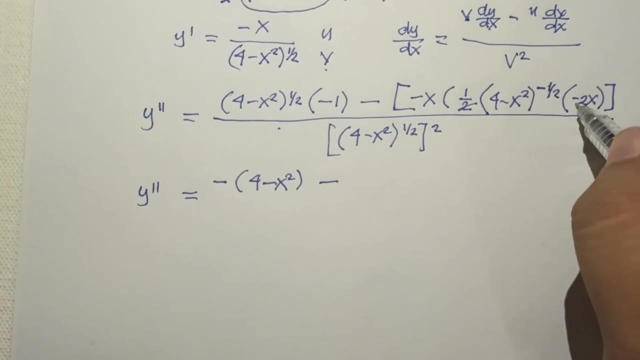 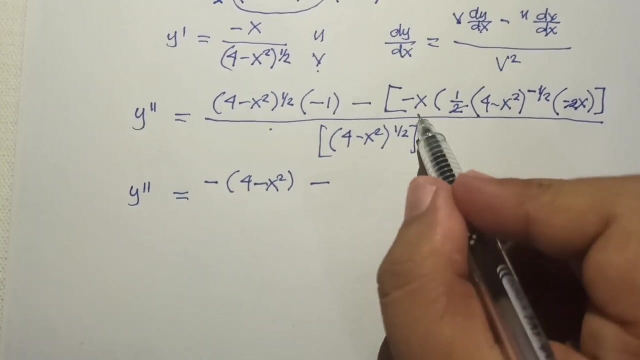 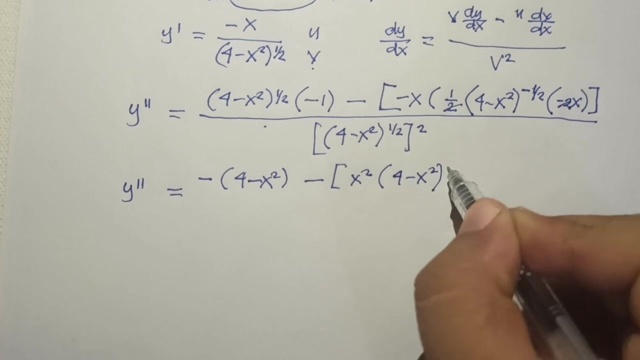 negative 4 minus x squared minus. so cancel this part, cancel 2.. So negative divided by negative, that is x negative x times negative x. the result is x squared times 4, x squared copy raised to negative 1 half Over this: 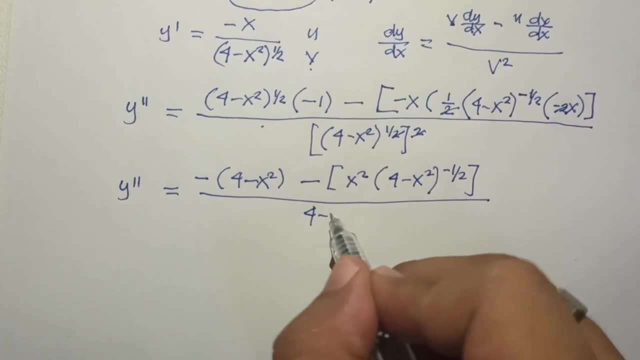 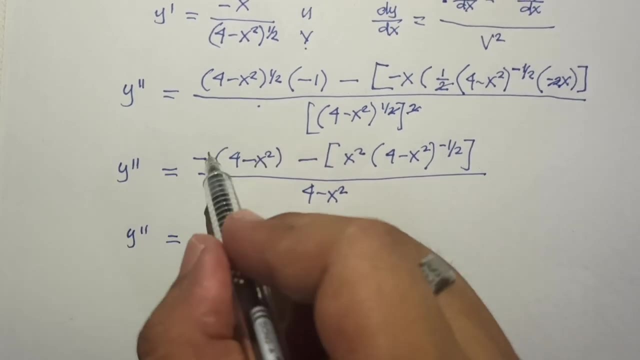 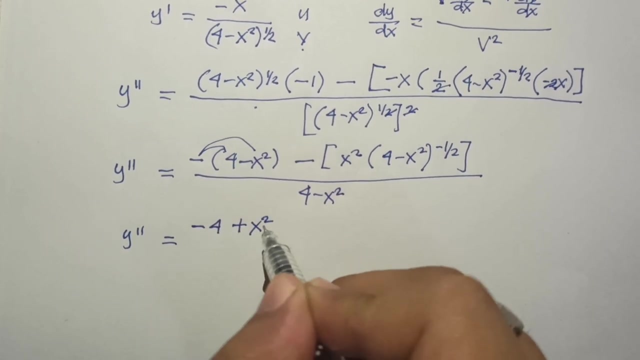 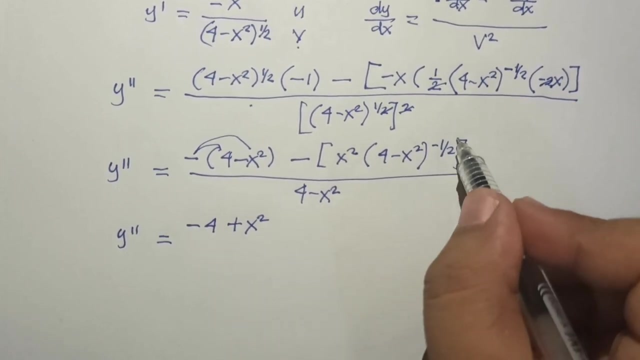 This cancel part. so therefore we have 4 minus x squared, So double prime. so we need to distribute the sign. So negative 4 plus x squared. So this could be expressed as: since this is negative, so we could have the exponent. 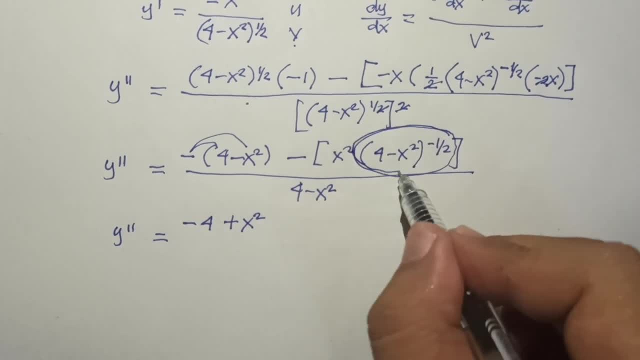 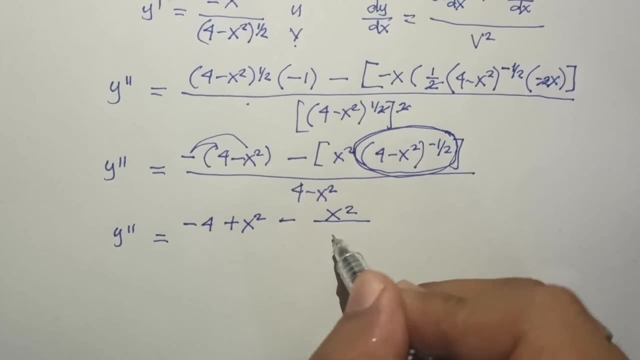 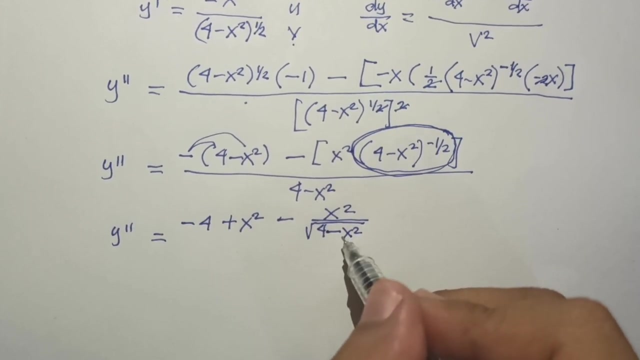 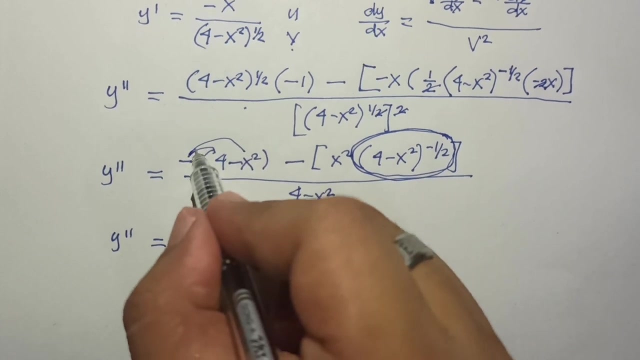 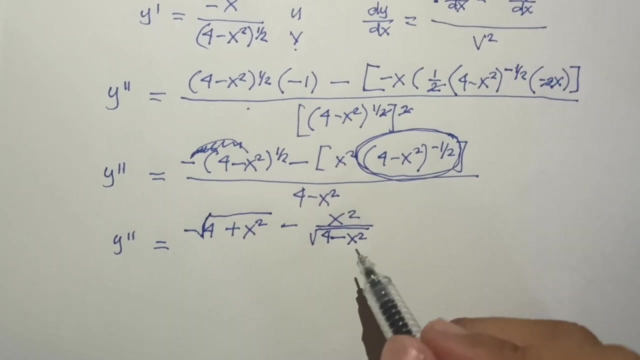 of this one radical will be in the denominator sign. so minus x squared over 4, or the square root of x squared, this is raised to 1 half Allah, although we cannot distribute sign because this is 1 half, so this is negative. this is the square root of. 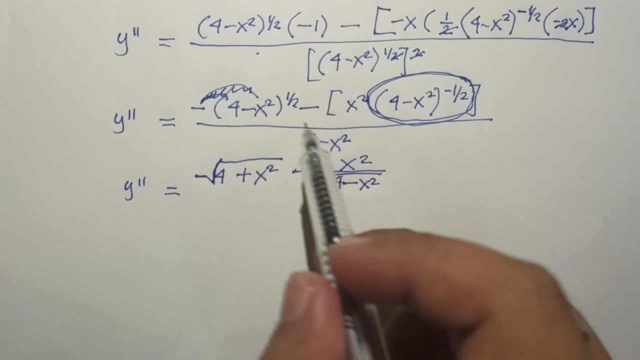 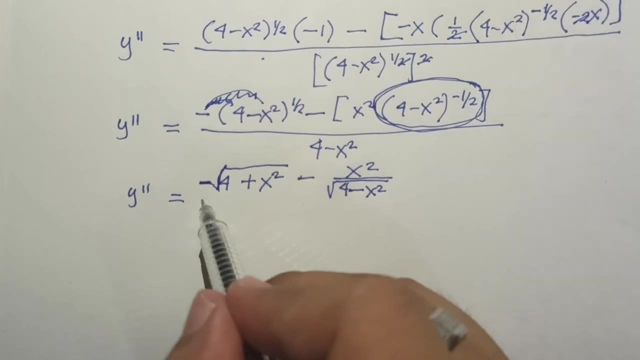 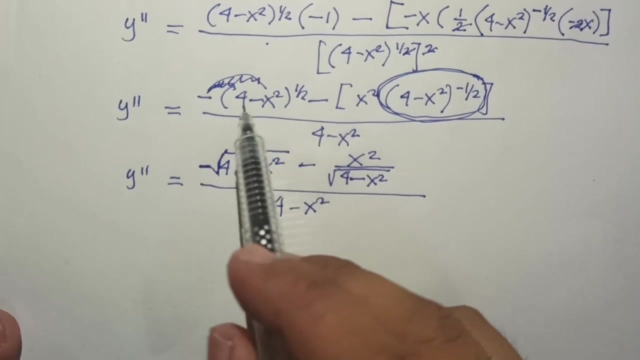 negative: square root of 4 plus x squared. I forgot to write the 1 half, so therefore we have negative the square root of 4 plus x squared over 4 minus x squared. so the little upon at the equation again. so we could not distribute because still we have the 1 half, but we could express it 1 into a radical. 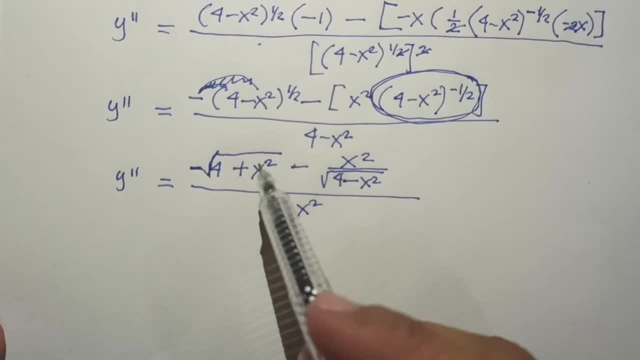 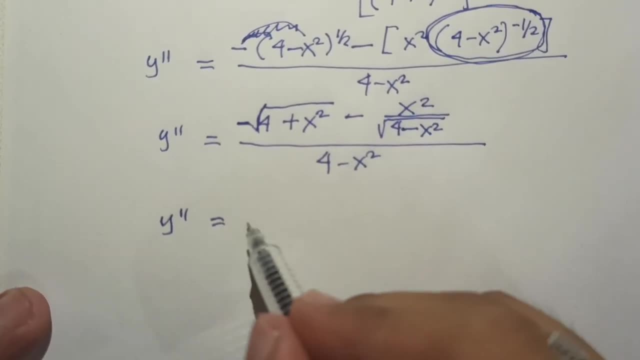 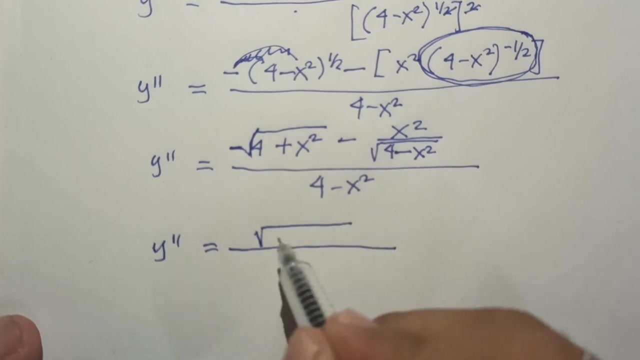 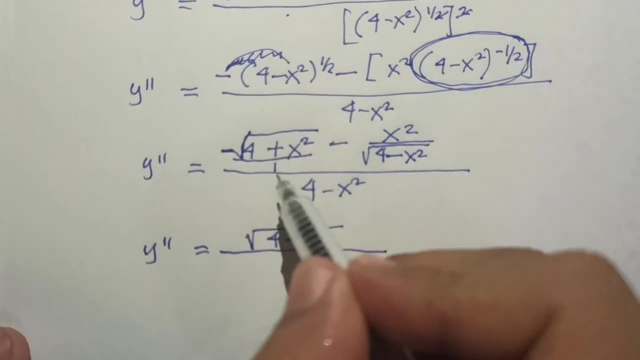 radical terms. ok, taken square root of x, so double prime is equal to. so we need to take the LCD, the LCD of this one, your square root of 4 minus x, squared so for and understood. we have a one here. so an every fraction arrow number, we 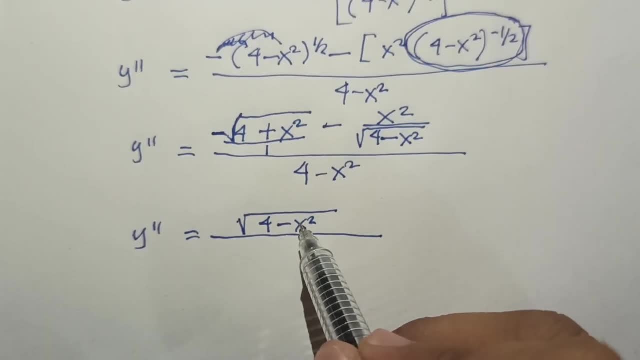 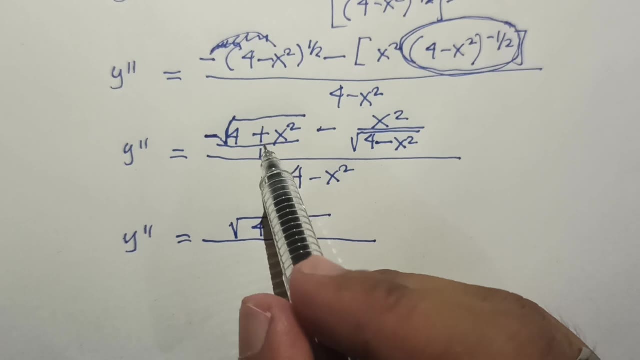 have over one. so square root of 4 minus x squared divided by 1 is still the same square root of 4 minus x squared times this part. so like the square root. so because 1 half plus 1 half, that is raised to 1. 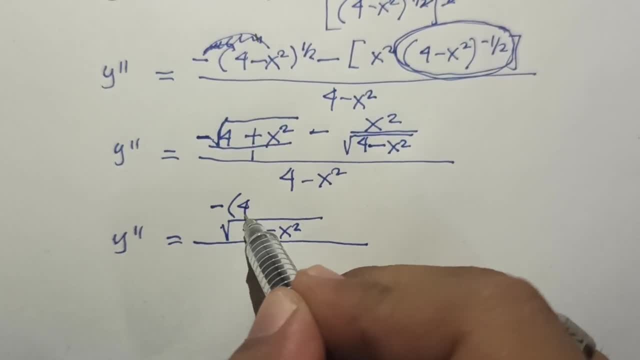 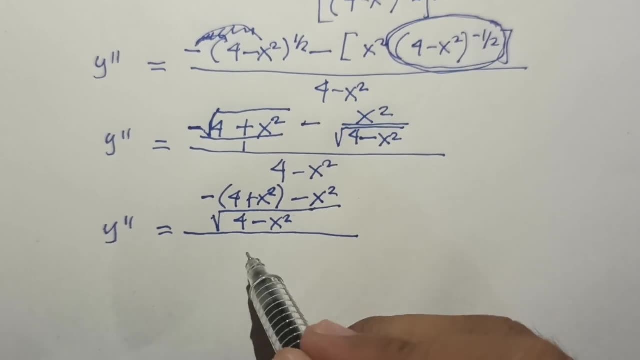 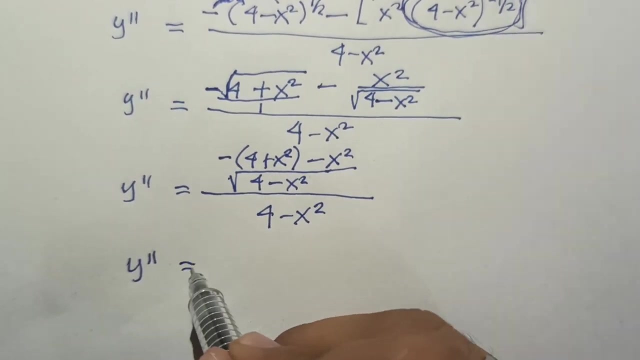 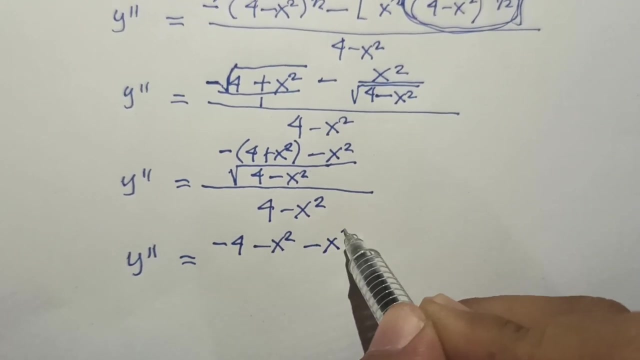 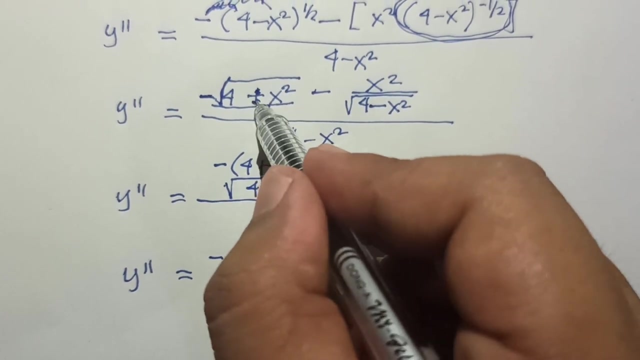 so, therefore, negative: 4 plus x squared, minus x squared. and we have here the denominator which is 4 minus x squared. so we need to simplify. okay, in simplifying, we have negative: 4 minus x squared, minus x squared. okay, i, this is negative. so this, this is negative based on this part. 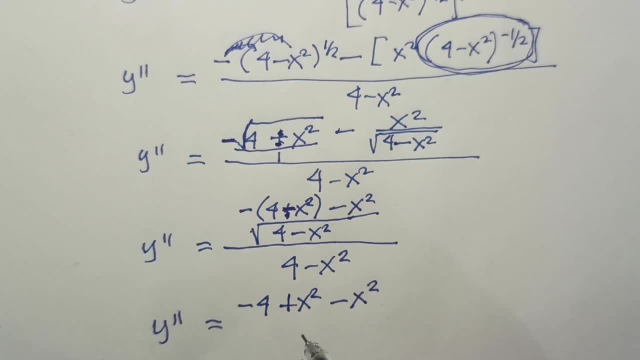 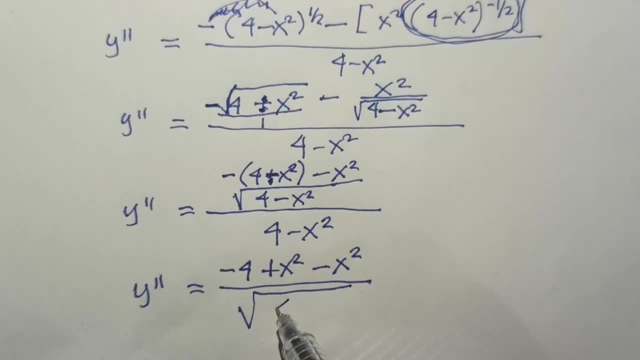 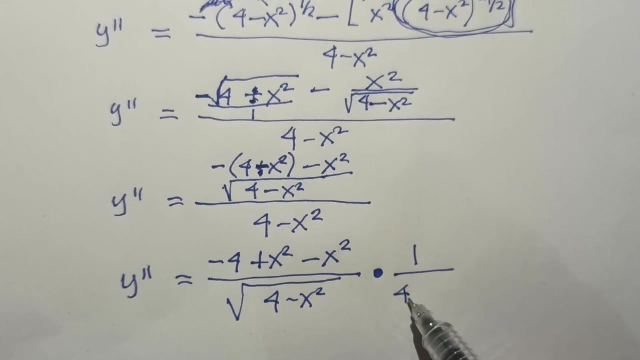 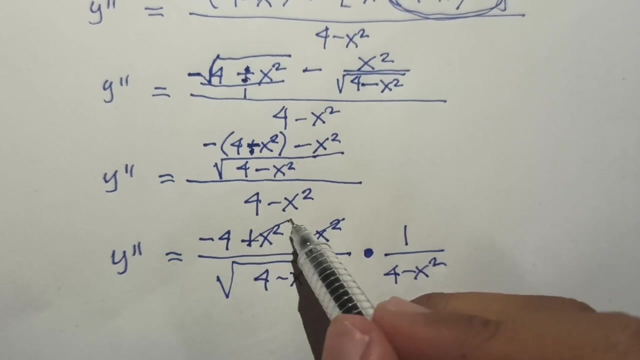 so this is negative. so this is positive over the square root of 4 minus x squared. and we need to take the reciprocal of this one, 1 over 4 minus x squared. okay, so cancel this part. so y double prime is equal to negative 4 over. 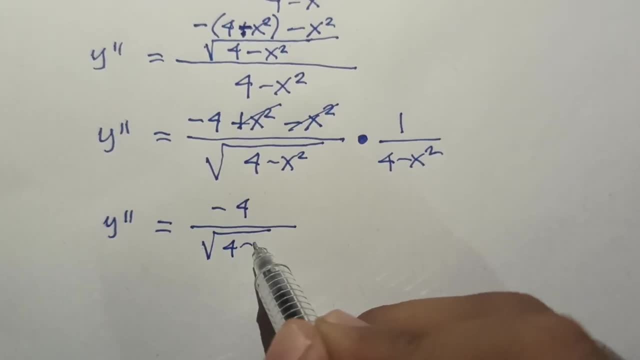 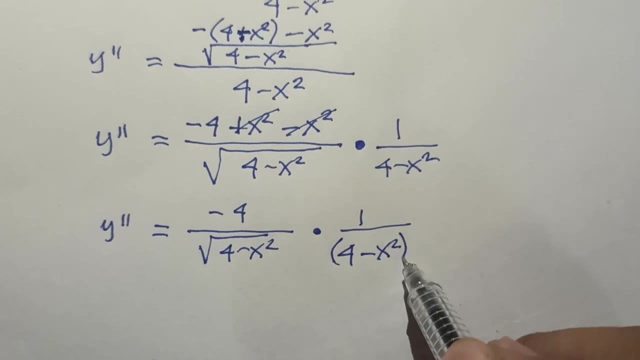 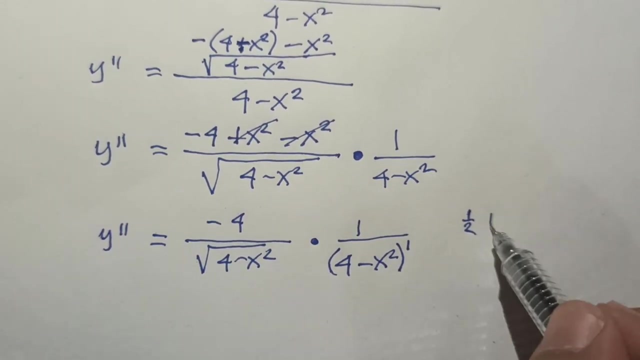 the square root of 4 minus x squared times 1 over 4 minus x squared. so we have negative 4 minus x squared times 1 over 4 minus x squared. so we could still raise this one as 1, so therefore 1 half. this is 1 half because this is square root plus 1 because 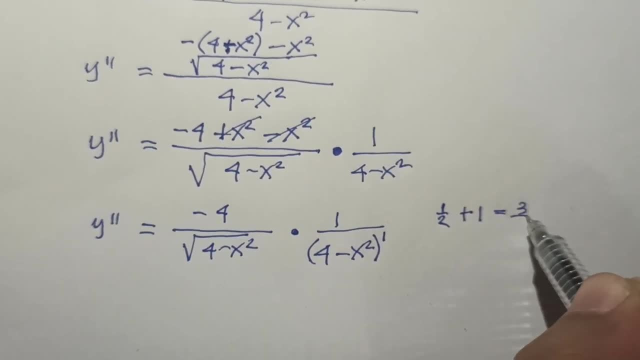 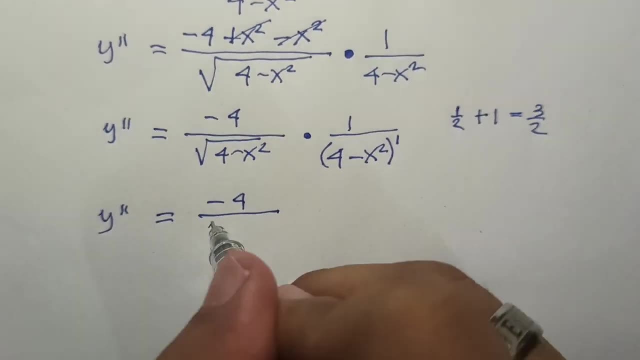 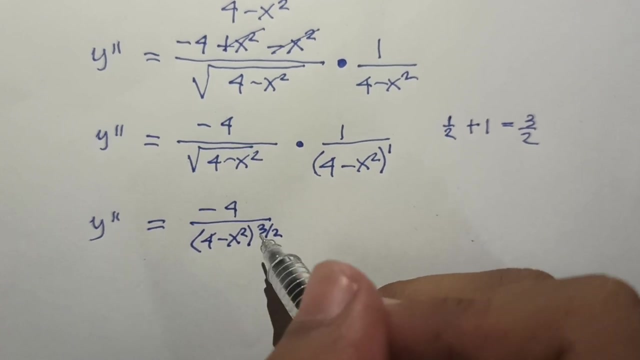 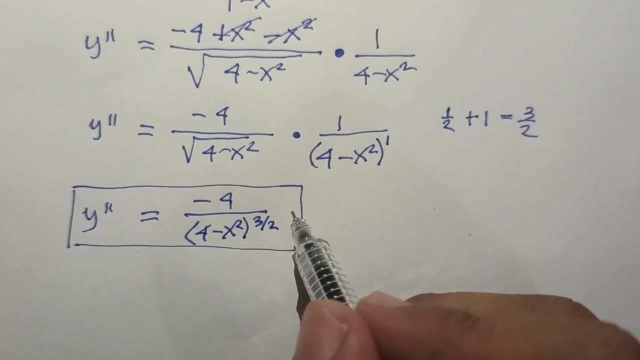 you're multiplying plus 1 is equal to 3 half. so therefore y double prime is equal to negative 4 over 4 minus x, squared raised to 3 half. so we can have this, this one, as the second derivative. okay, so in order for us to get the third derivative, we could. 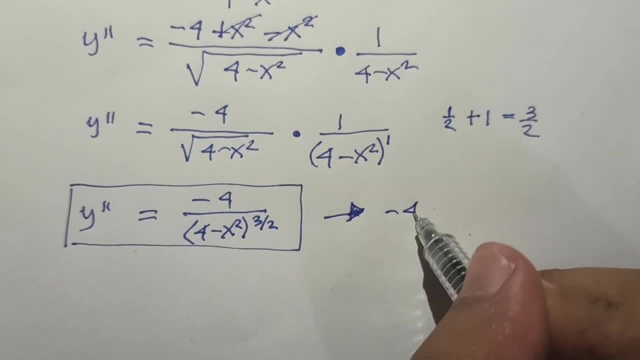 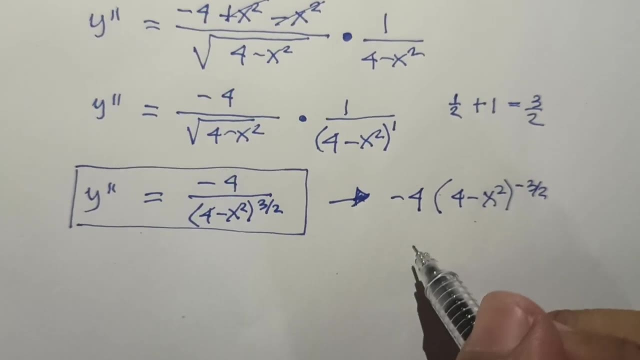 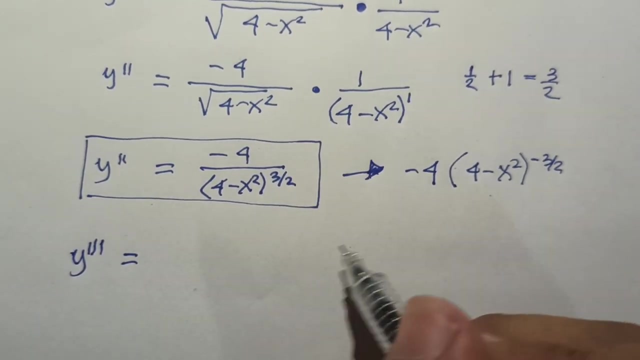 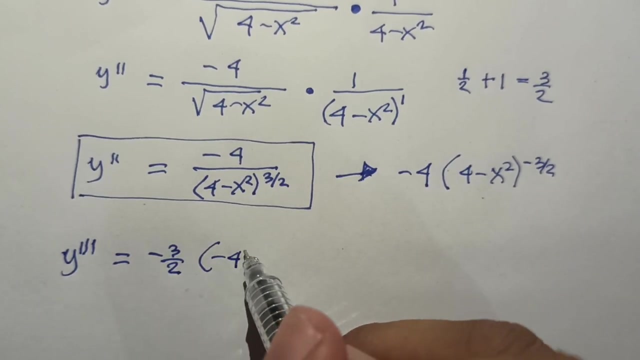 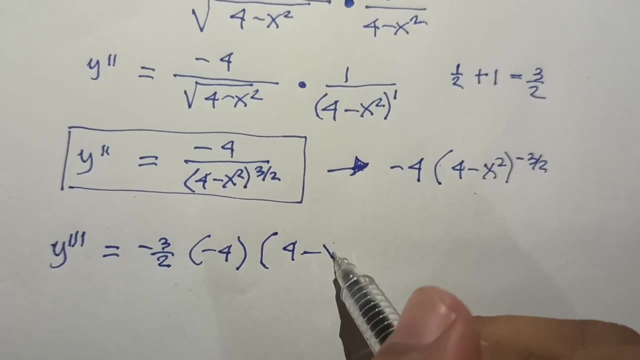 express this one as negative four, then times four minus x, squared, raised to negative three halves. so in order to get the third derivative we have to express: so negative three halves times negative four times four minus x, squared, then derivative of the u based on the chain rule. 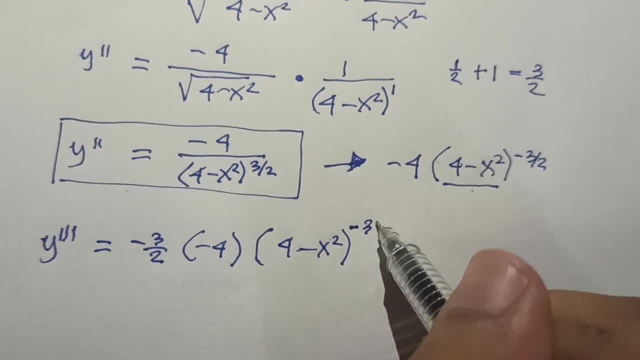 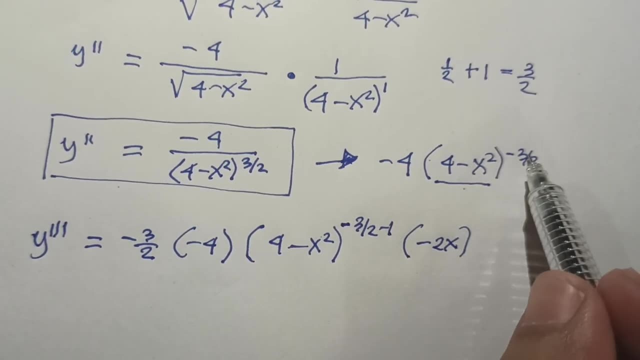 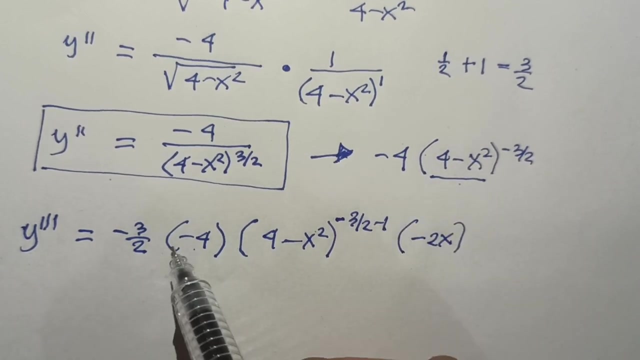 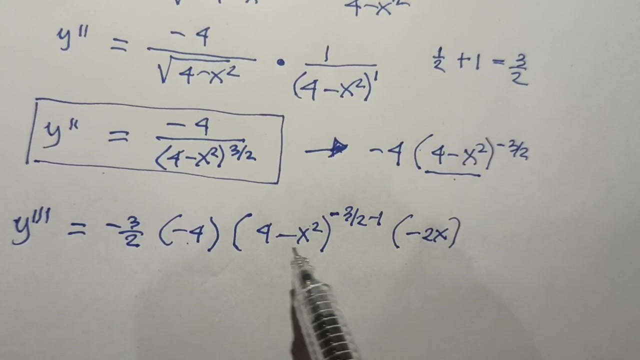 uh, negative three halves minus one, plus times the derivative of this part. we have two x going back. negative three halves times negative four. bring down right the. take the product of this one and copy the u, which is four minus x squared, and negative three halves minus one and the derivative of u, which is: 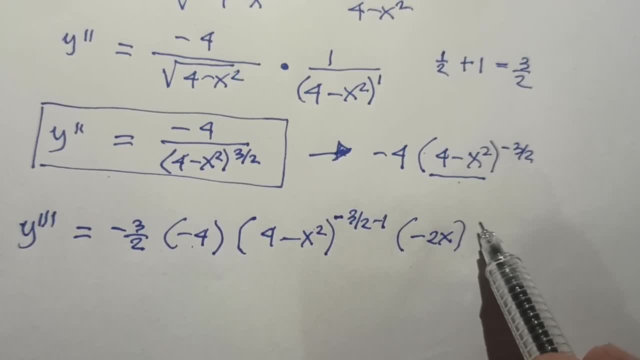 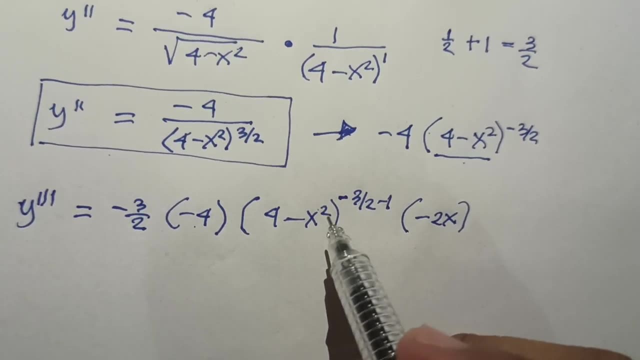 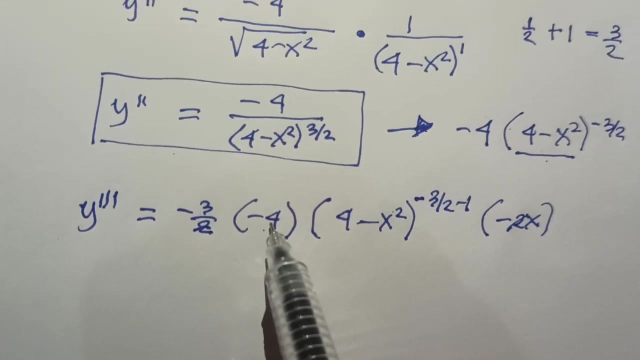 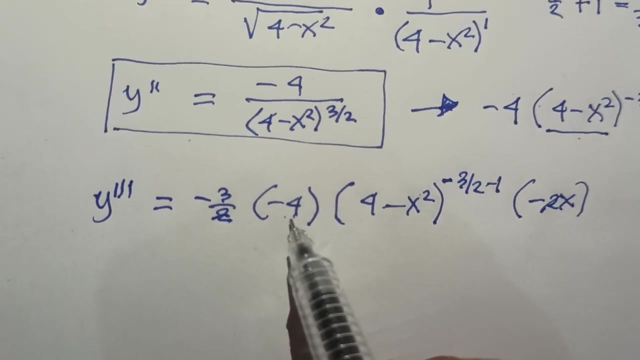 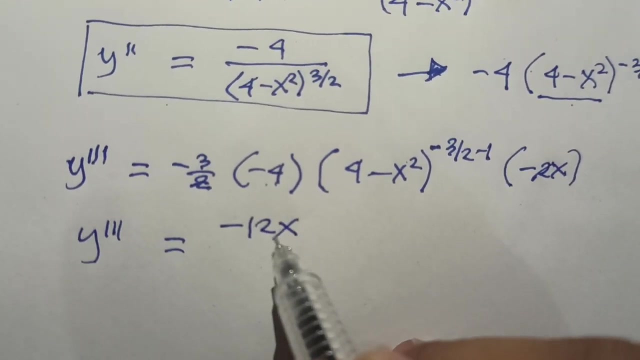 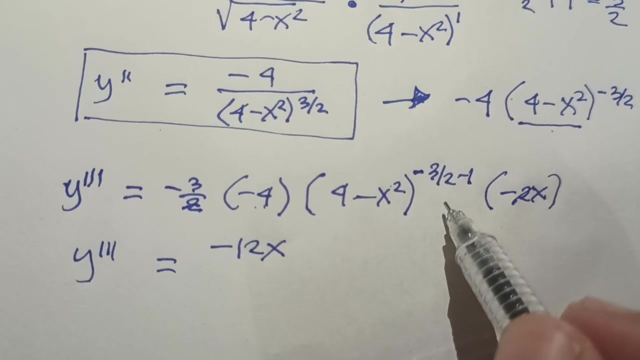 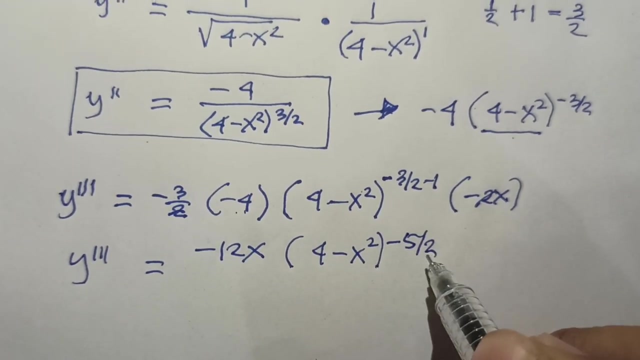 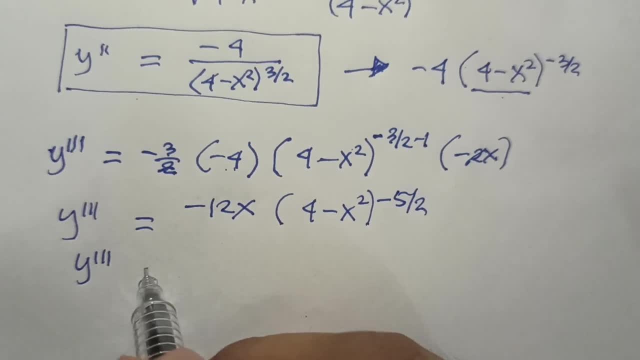 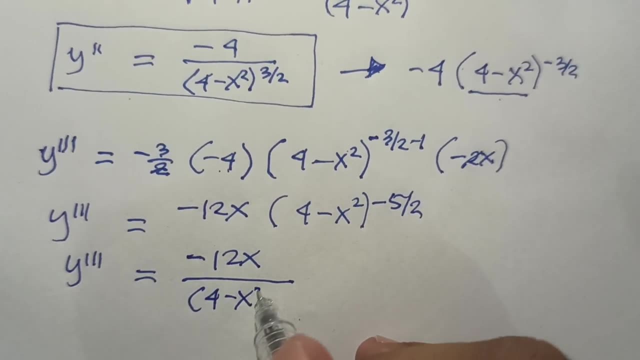 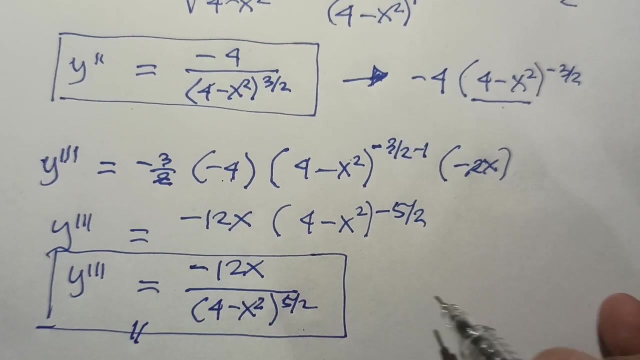 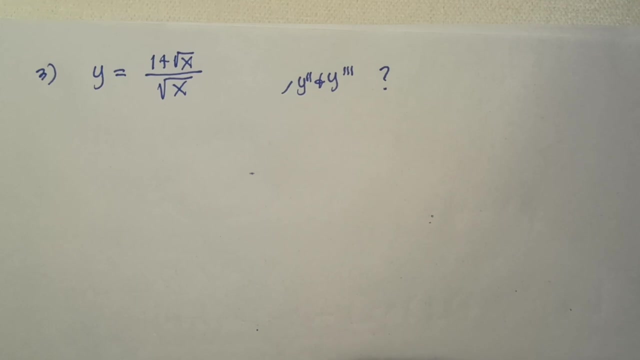 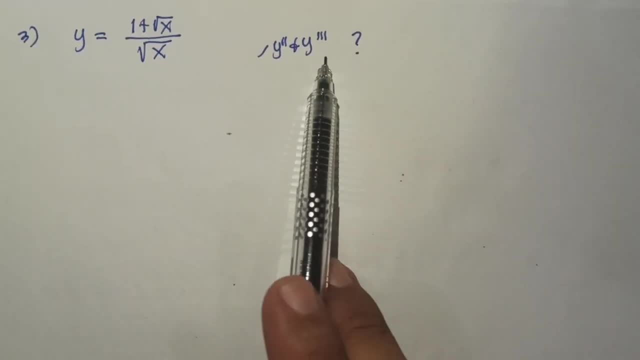 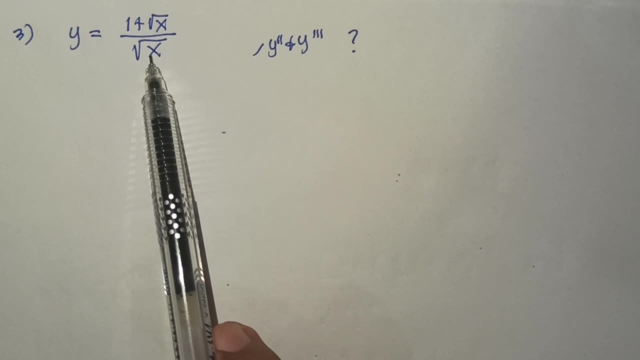 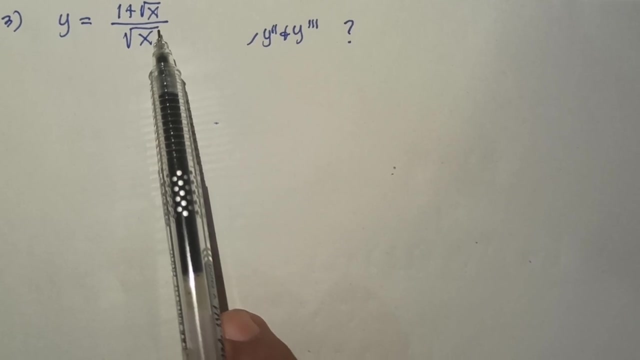 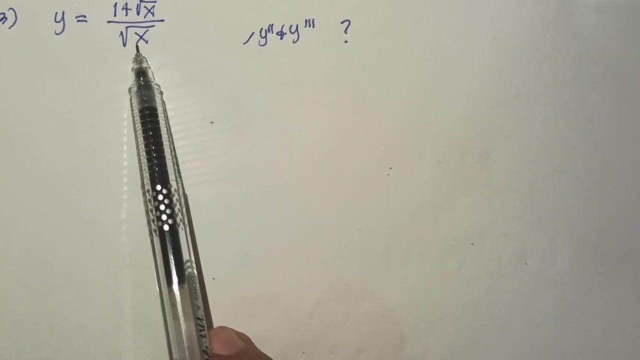 we need to find the second derivative and the third derivative. so the trick here is we need to place this one into the numerator and express these all terms into a fractional form. so instead of radical, we need to transpose this, or express this one into radical to have an easy differentiation. so let's try so Y. 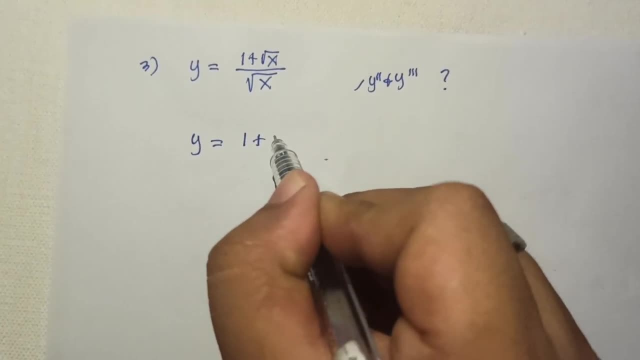 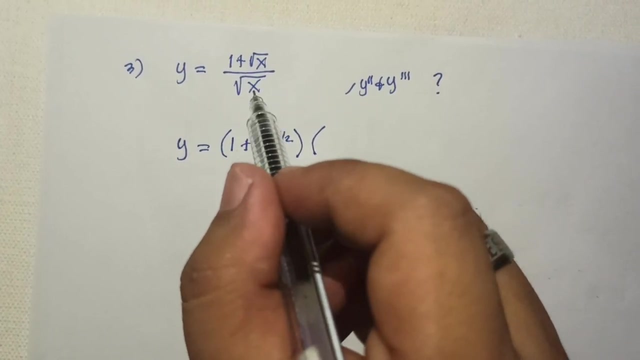 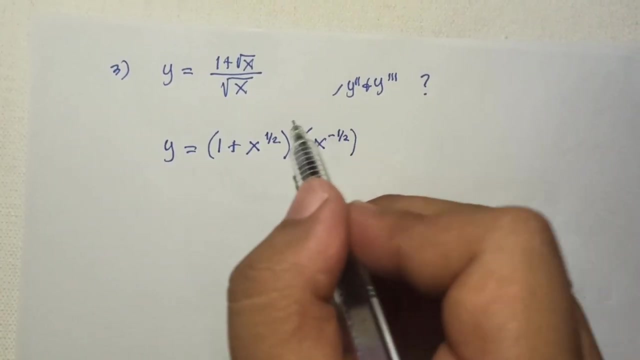 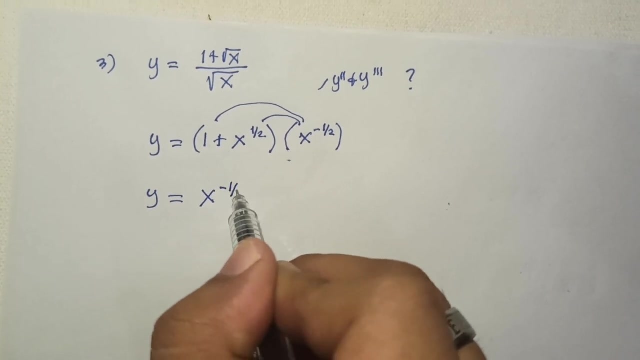 is equal to 1 plus X raised to 1 half times. so since this is a square root and this is denominator, the result would be X raised to negative 1 half and you have to distribute this part. so Y is equal to X raised to negative 1 half. 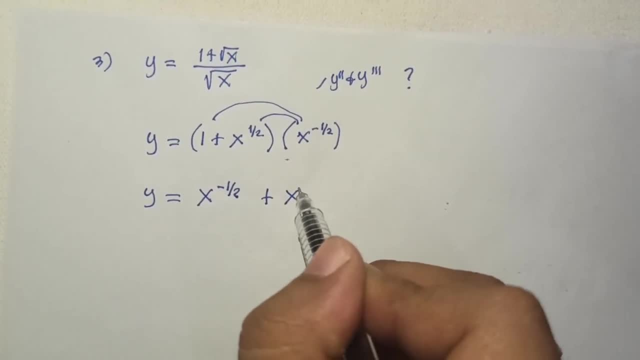 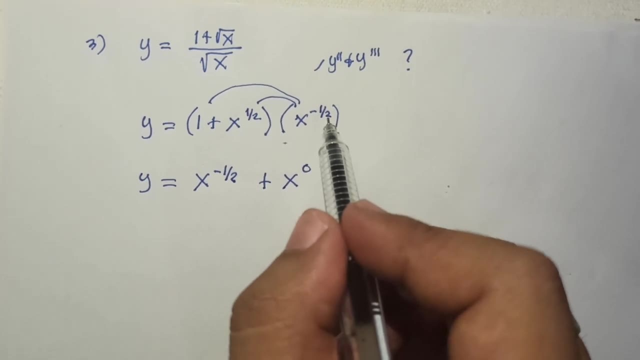 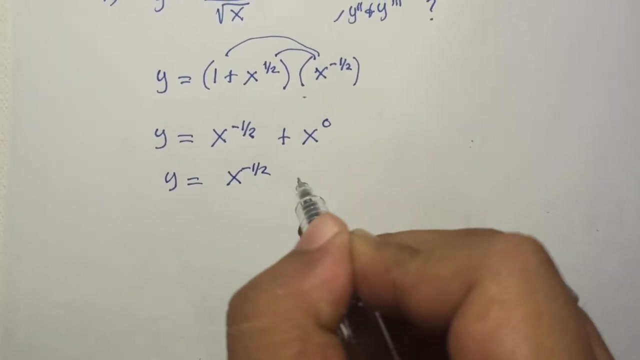 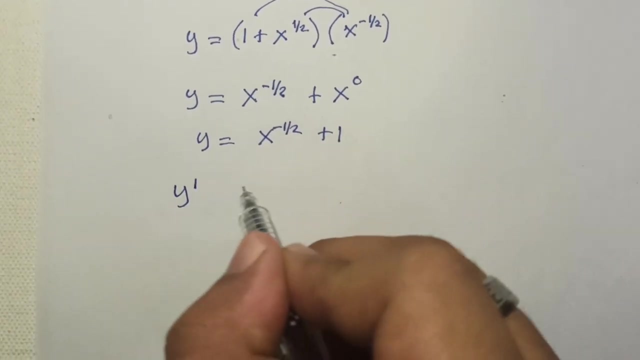 plus X raised to 0, write one half plus negative 1 half nerve of exponent based on the loss of exponent. so therefore, x raise to 0, Y is equal to x raised to negative, 1 up plus 1 key. so this is what we are going to differentiate in the first 3ating. so in 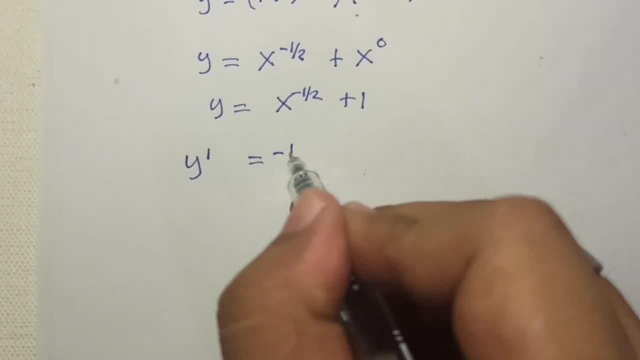 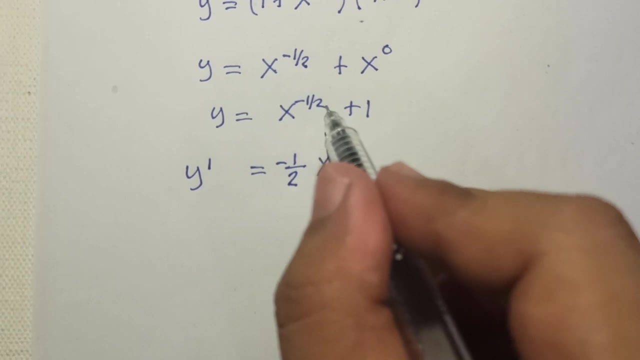 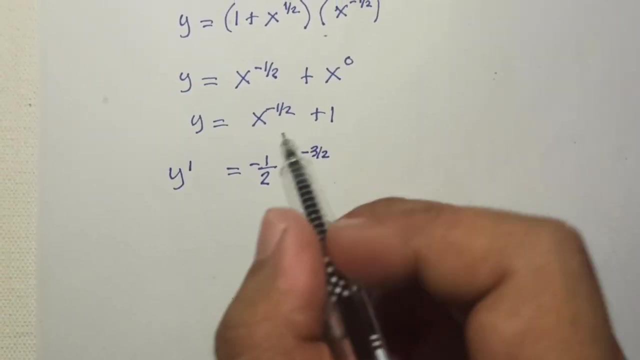 the first derivative. copy this part. so negative 1 half X raise to negative Negative one-half minus one, that is negative three-halves, And the derivative of this one is equal to zero. So that's why this is the first derivative, Okay. 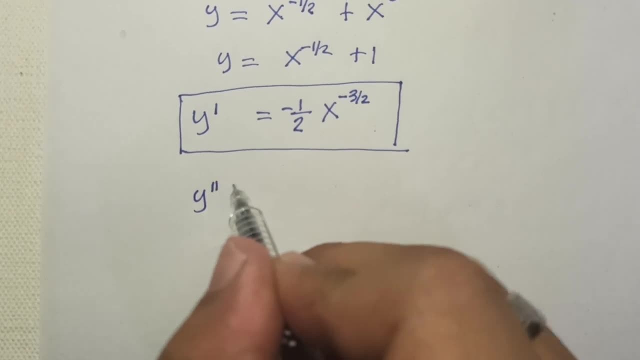 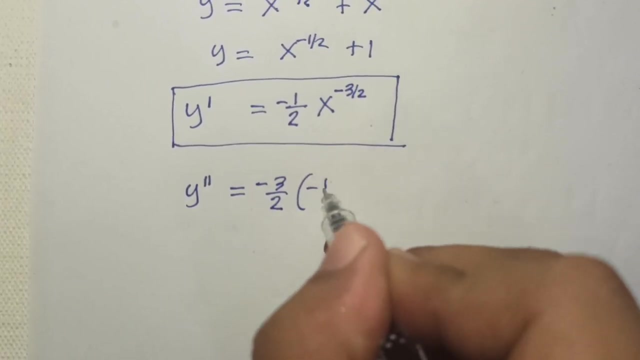 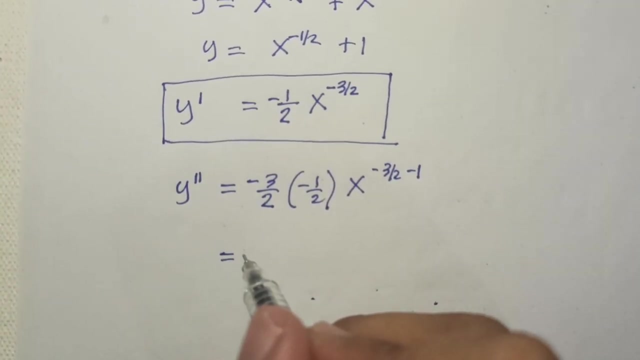 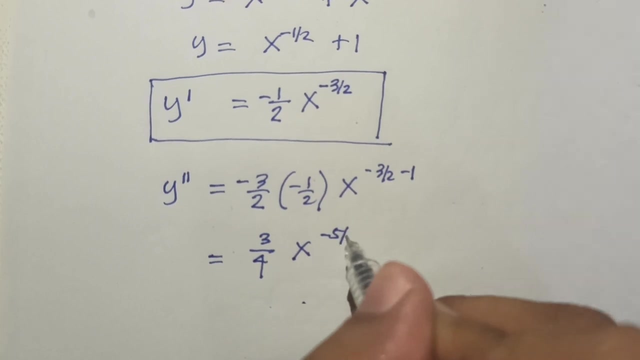 And to take for the second derivative. okay, so just take the derivative of the first derivative. So we have negative three-halves times negative one-half x raised to negative three-halves minus one. So we have the result is three over four x raised to negative five-halves. 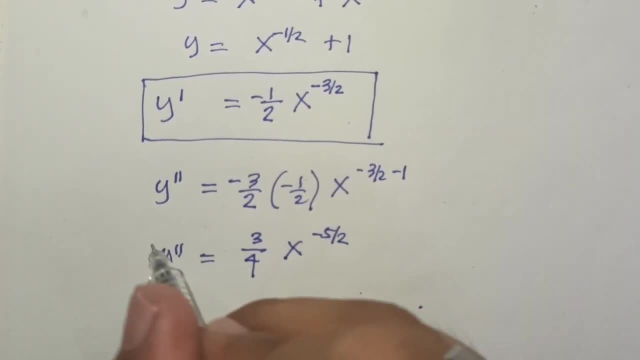 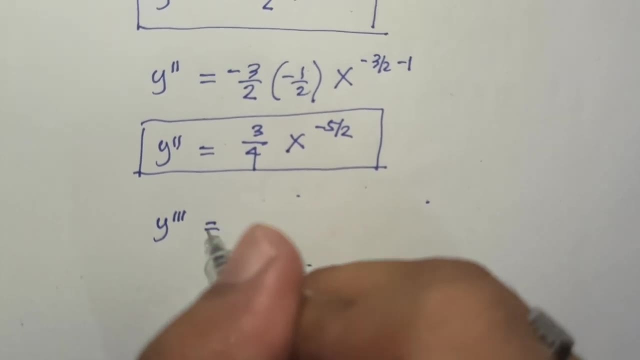 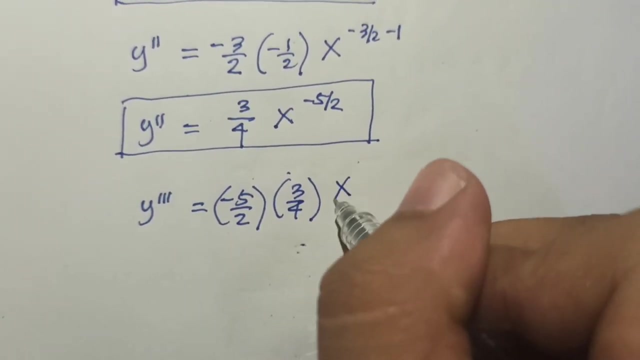 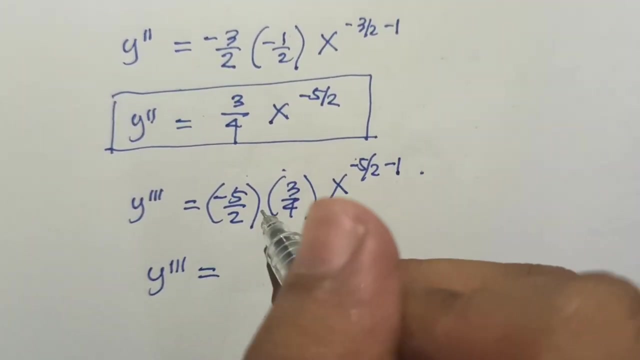 So this is the second derivative, And the third derivative is y triple prime. So negative five over two times three over four. x raised to negative five over two minus one. So triple prime is equal to negative fifteen over eight. x raised to negative seven over two. 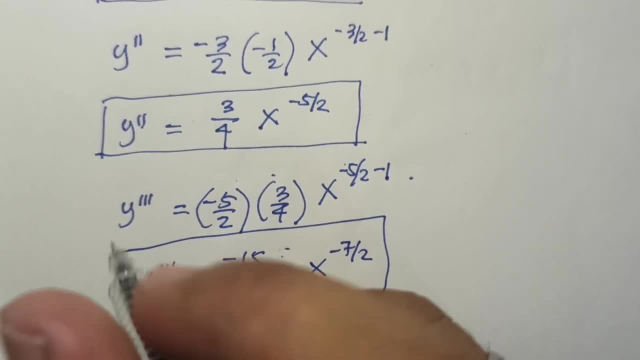 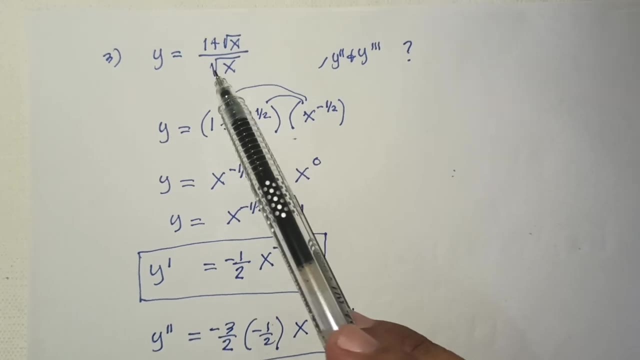 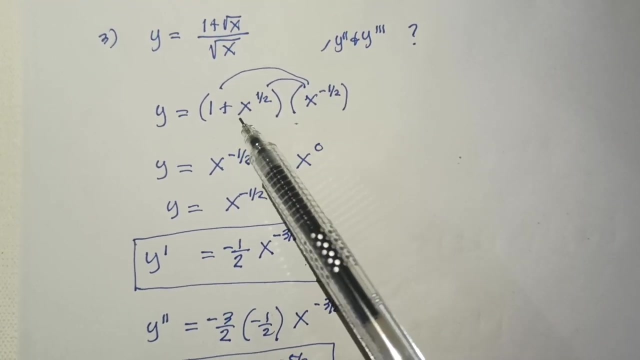 So this is the third derivative. Very easy, But as you look at the equation, it might be complicated for you too. And so, but the note is, we need to put that one in the numerator and express this one into a fractional form. 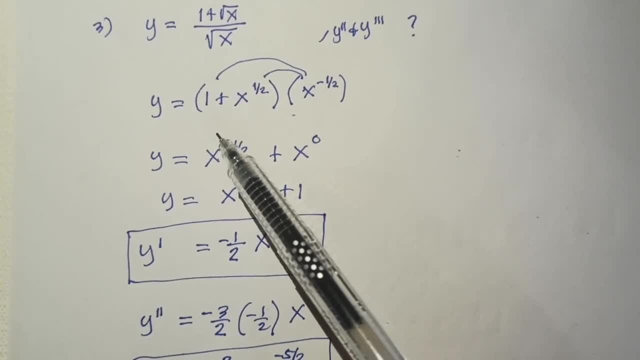 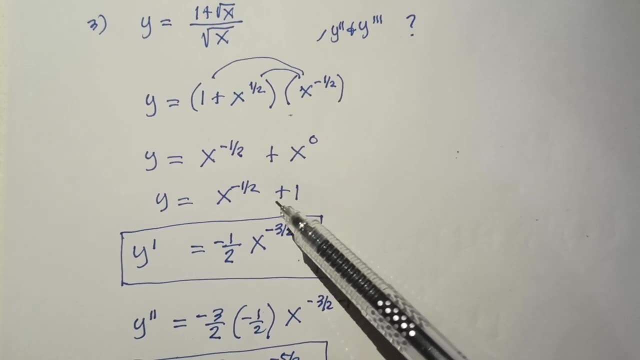 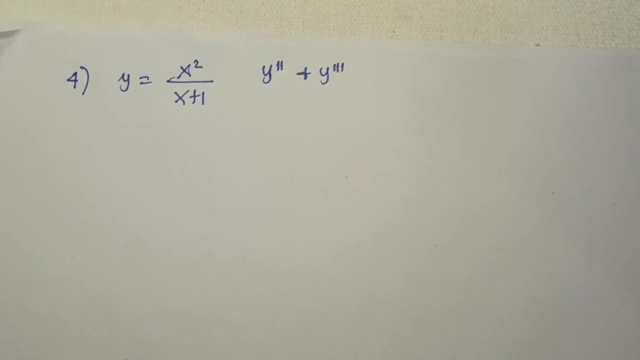 Express into an exponent of a fractional form, For you have an easy way of differentiating and simplify first before you are going to differentiate. So that's all about number three. Okay, So we are now in number four. Okay, So y is equal to x squared over x plus one. 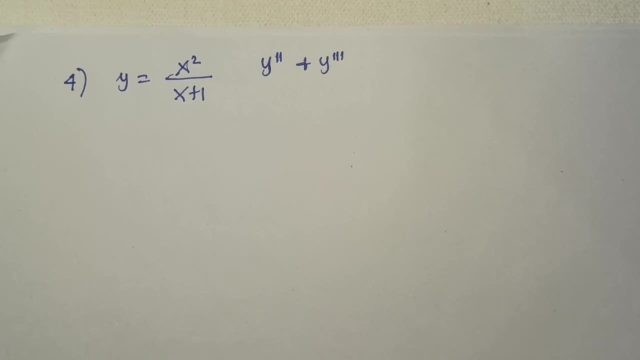 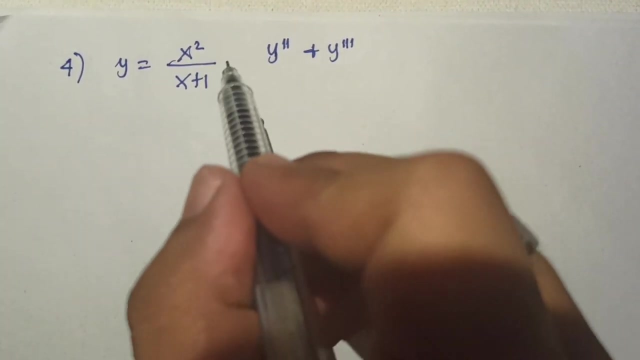 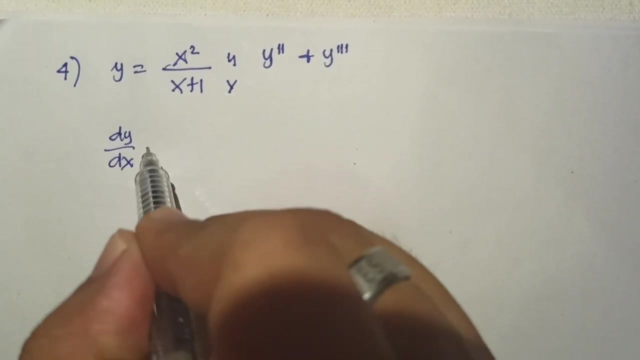 So in this case, we need to find the second again and the third derivative. So in this case, so this is in the form of a quotient rule. So therefore, this is our u and this is our v. So going back, so dy over dx is equal to v, du over dx minus udv. 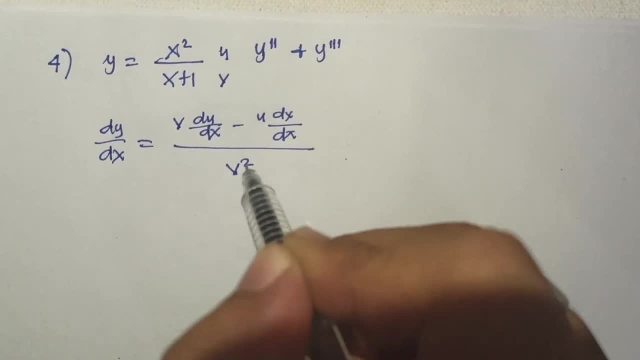 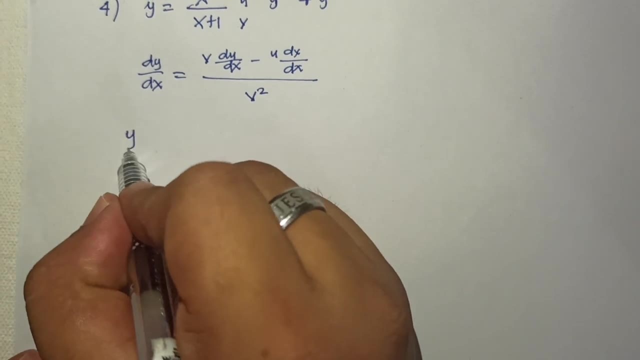 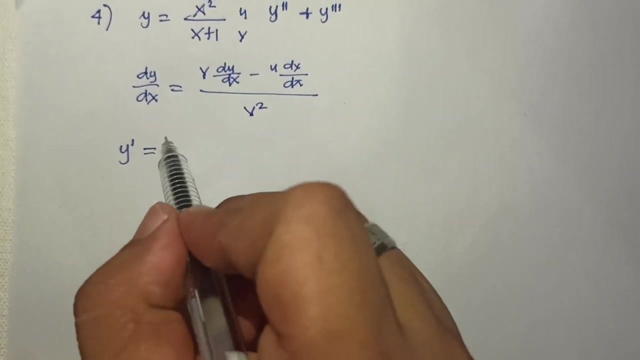 Over dx over v squared. So did I forget this formula: v du minus udv over v squared. So first take the first derivative. So first is copy the v. So just copy the x plus one And you need to take the derivative of u, which is x squared. 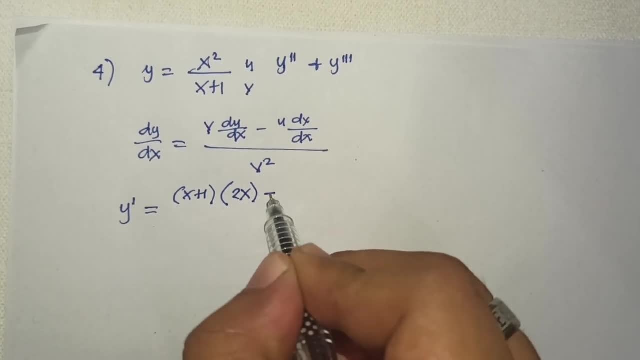 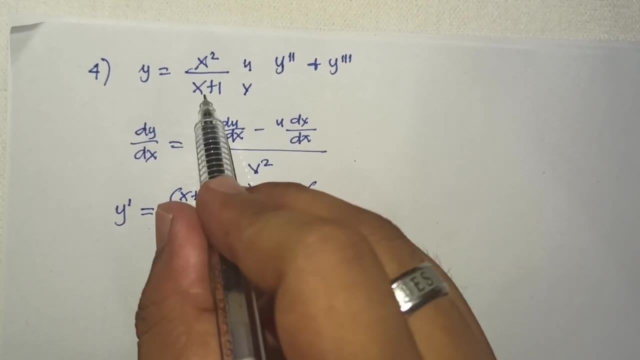 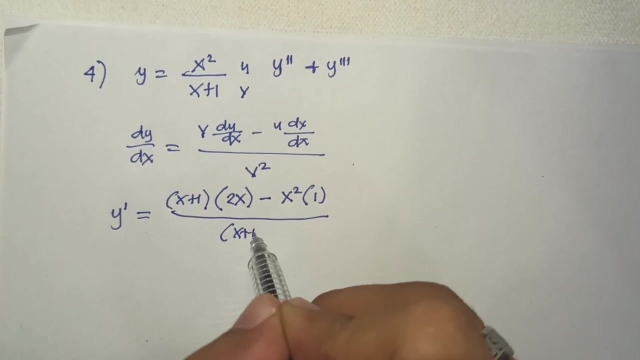 The derivative is 2x. Just follow the formula And Copy the u, which is x squared, And the derivative of this one is equal to x plus one is equal to one over v squared, which is x plus one squared. So y prime is equal to distribute. 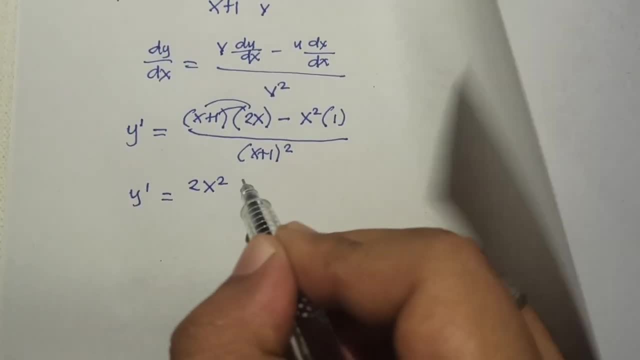 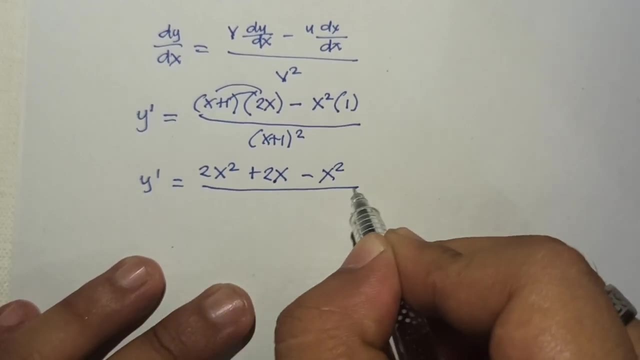 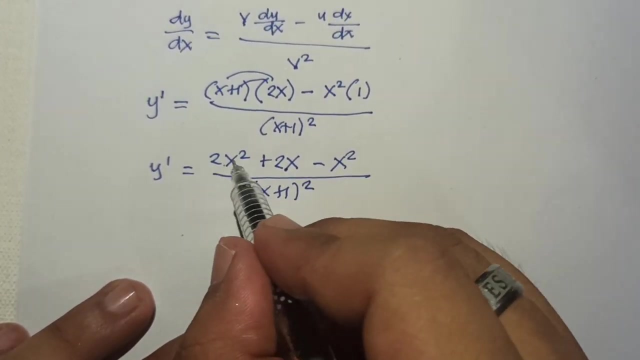 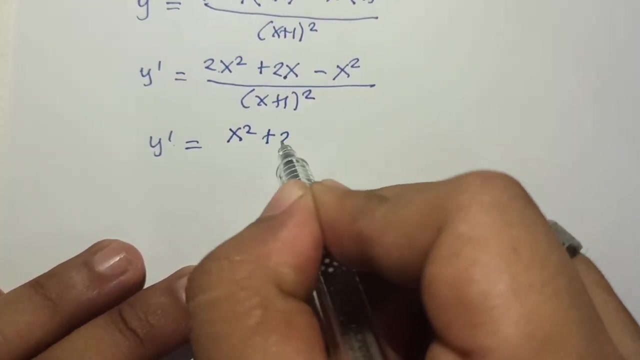 So therefore we have 2x squared plus 2x minus x squared over x. So y prime is equal to 2x plus 1 squared. Okay, So 2x squared minus x squared, The result is x squared. Then copy: 2x over x plus 1 squared. 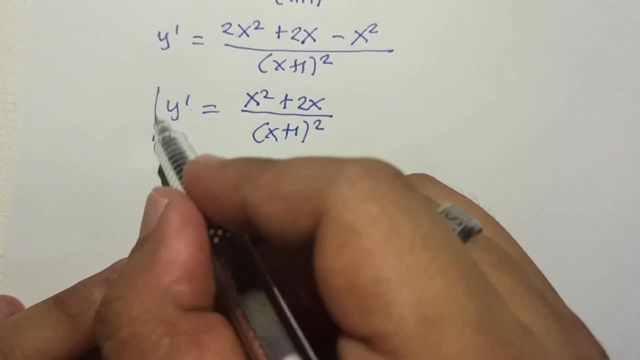 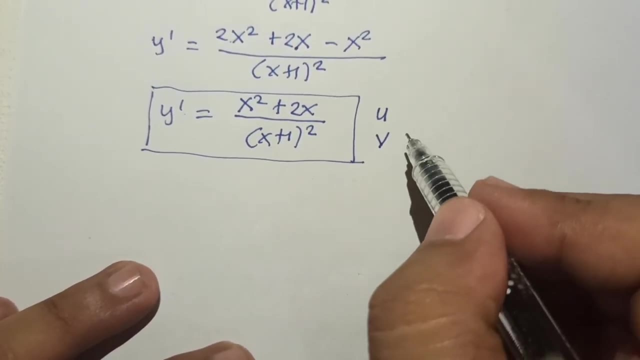 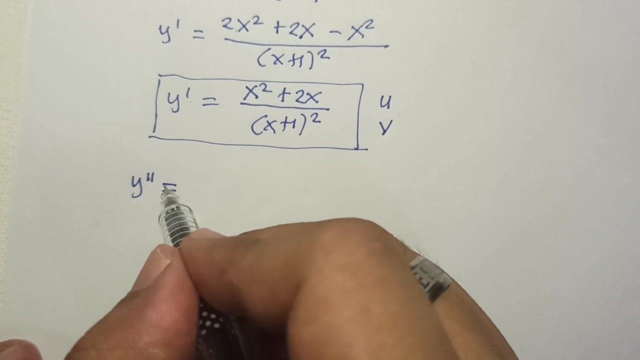 Okay, So this is the first derivative. So in order to get the second derivative still, you need to follow the u over v. So again, so y double prime is equal to v. so the formula is v du first v. copy x plus 1 squared. 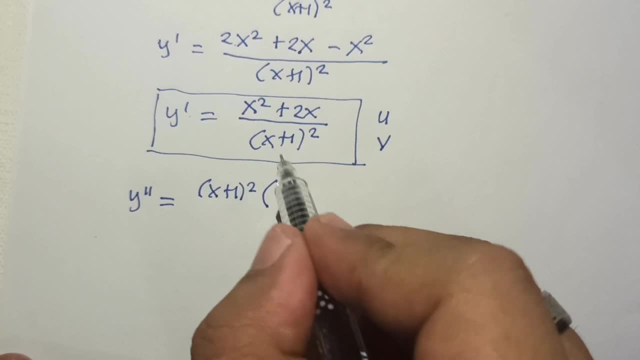 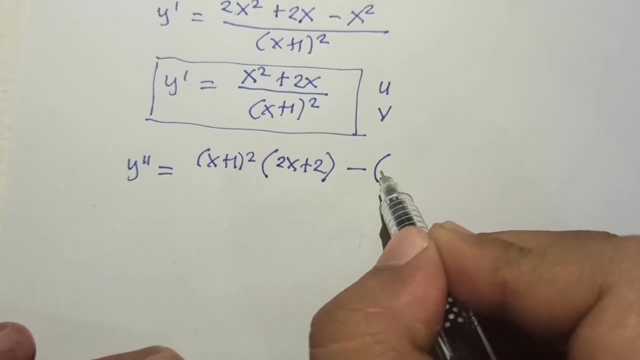 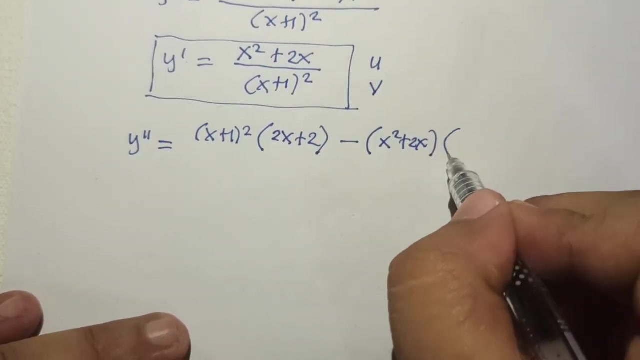 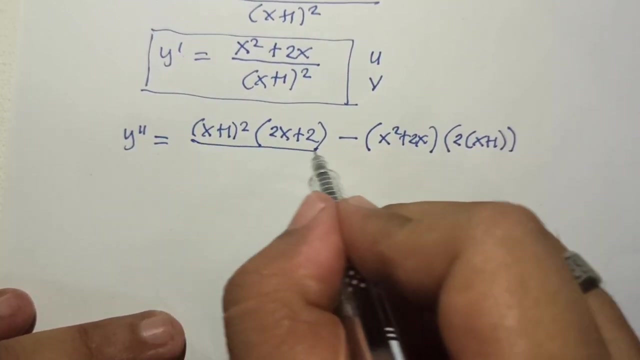 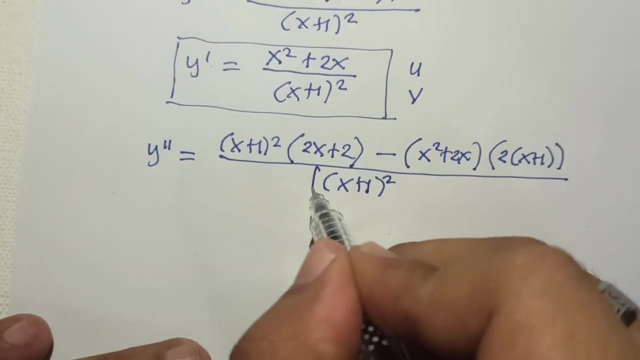 times the derivative of u, which is x squared plus 2x, that is, 2x plus 2 minus u. copy the u, which is x squared plus 2x, and the derivative of this one is 2 times x plus 1. okay, over x plus 1 squared, then you need to take the square, because v squared, okay. 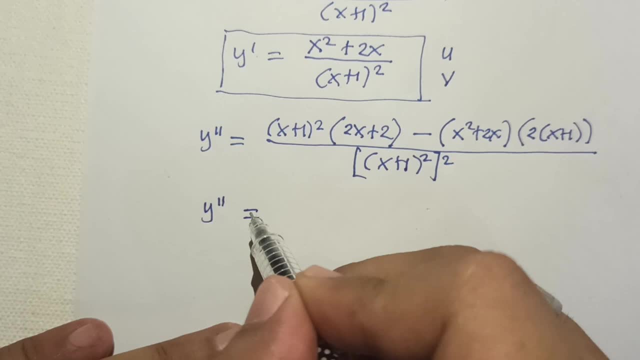 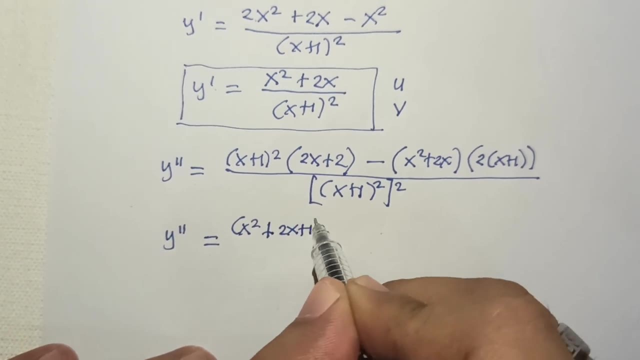 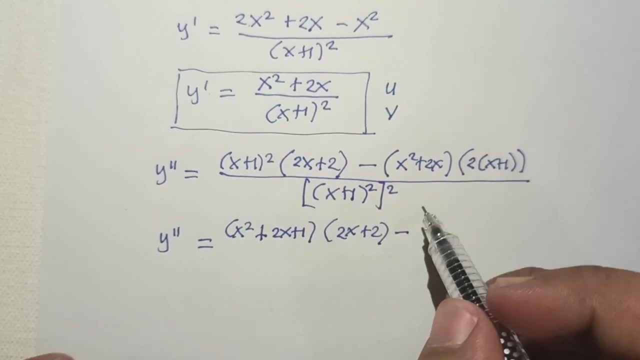 so y double prime is equal to v plus 1 squared times the derivative of u, which is x squared, so y double prime. we have to simplify first. so we have x squared plus 2x plus 1 times 2x plus 2 minus. we have to multiply this. 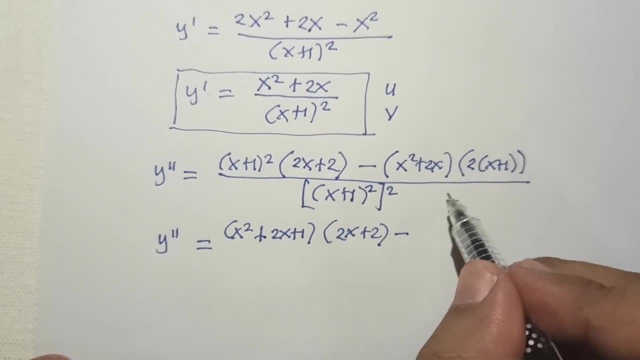 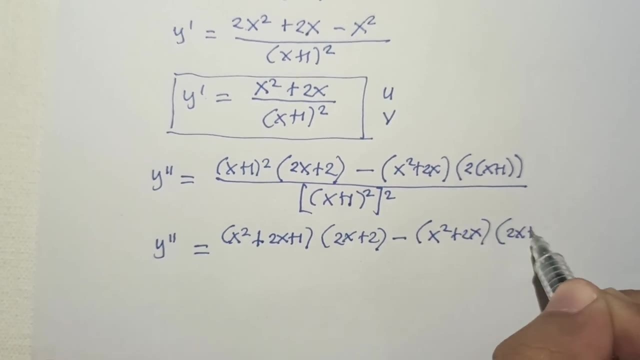 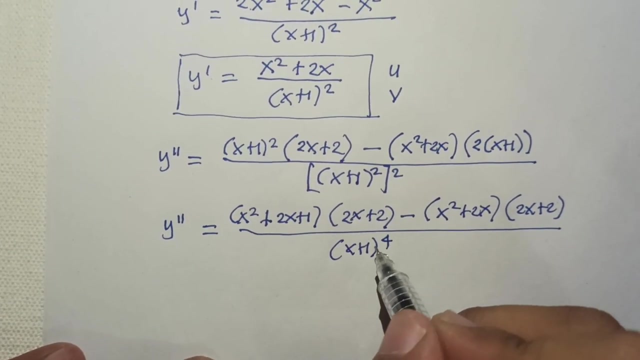 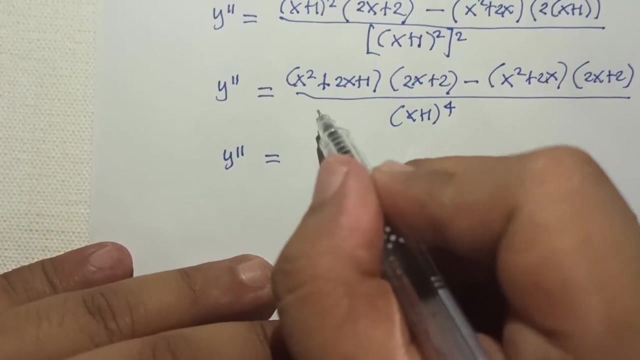 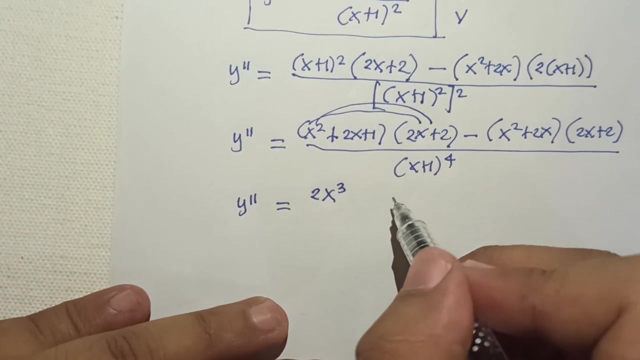 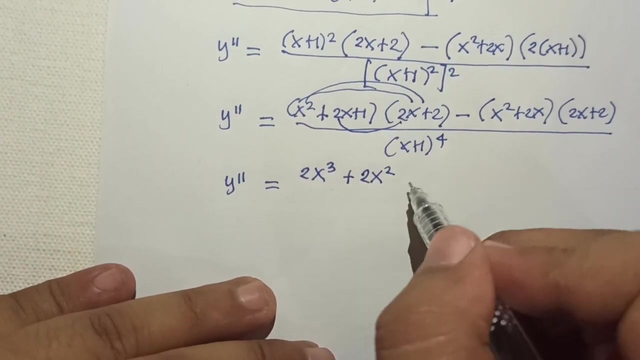 okay multiplying. so first simplify. so x squared plus 2x times 2x plus 2 over x plus 1 raised to 4. okay, so y double prime is equal to, so distribute this will become okay. 2x cubed plus 2x squared can distribute this part plus 4x squared. 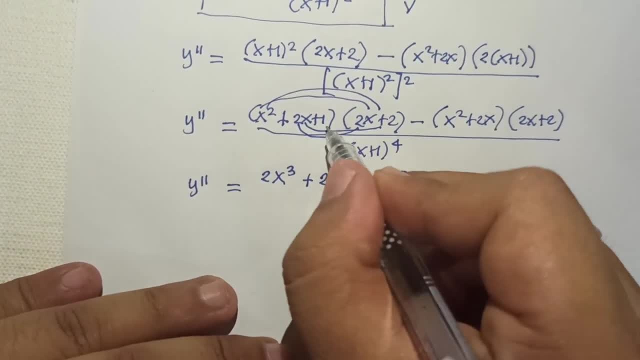 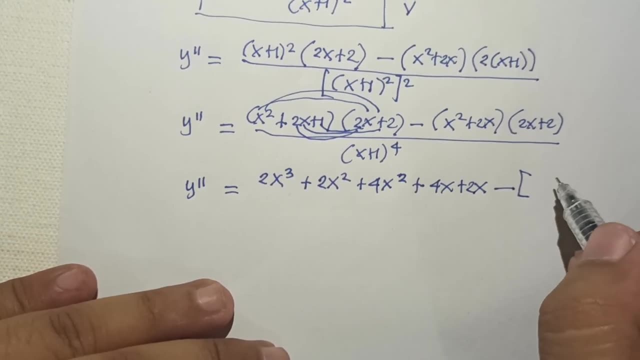 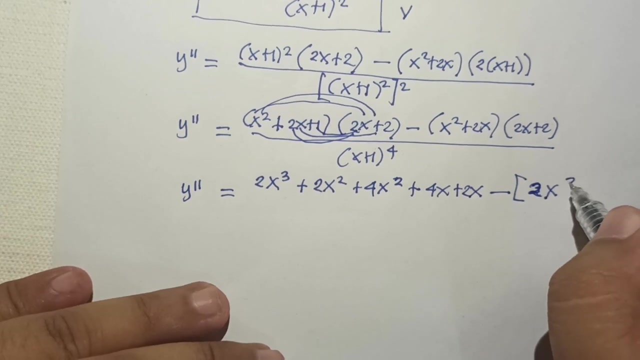 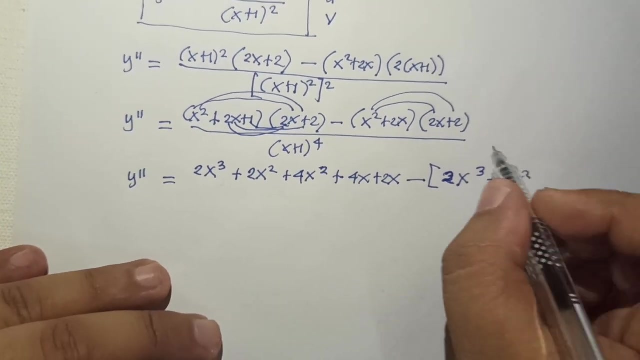 plus 4x plus 2x minus. we have distribute. we have 3, had 2 x-q first and a second plus 2x squared and this part plus 4x squared and this part 2x squared and this, okay, Cabライ dべ by repar 더 slowly from today. plus two times x squared plus 2x squared and this part plus 4x squared and this partches trabajar음. 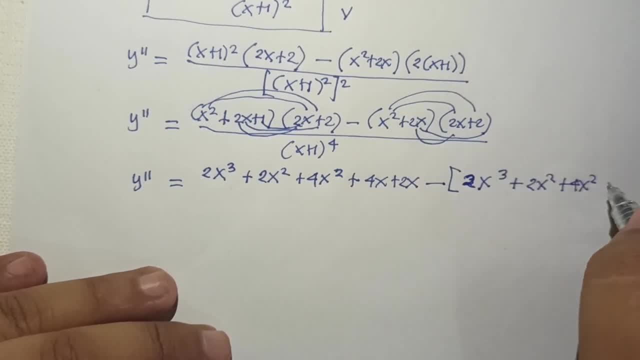 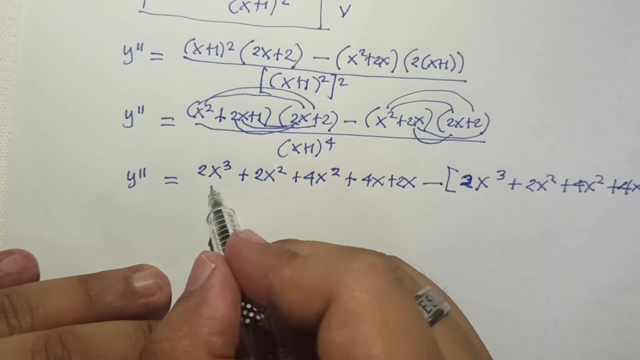 okay, y double prime is equal to v plus 1 squared than the derivative of u, which is x squared plus 2x squared times 2x plus 1 squared plus 2x squared and this partches and this part plus 4x. okay, over x plus 1 squared, okay. 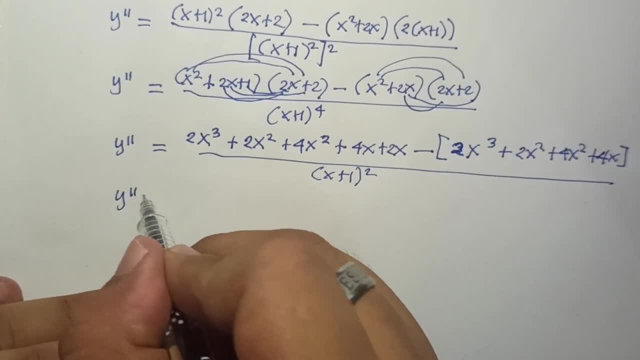 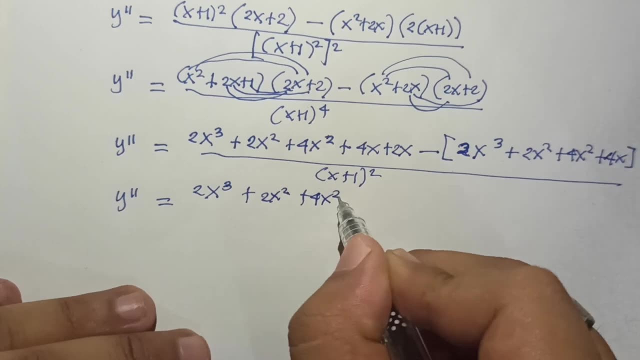 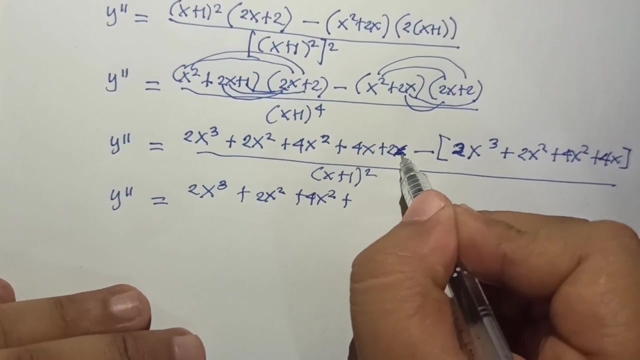 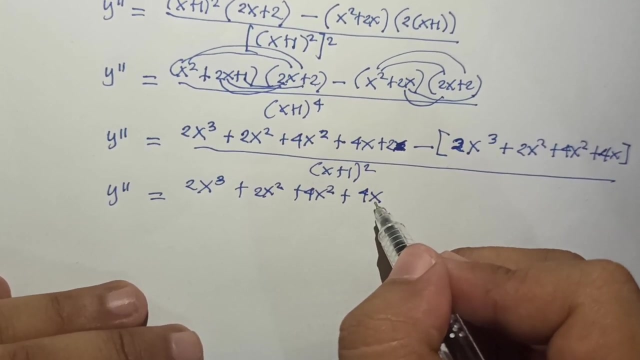 So we have simplify. how to simplify. so 2x cubed plus 2x squared plus 4x squared plus this is, by the way, this is 2, not 2x. okay plus 4x. okay. let's go back here. 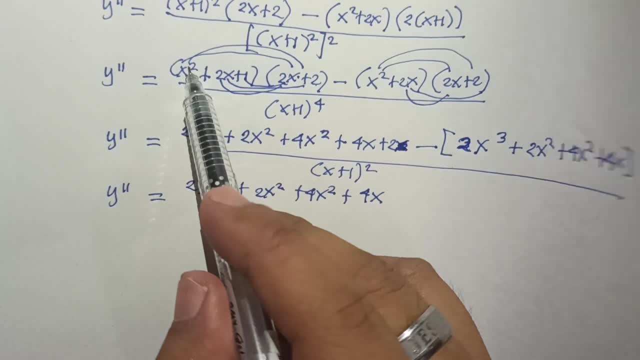 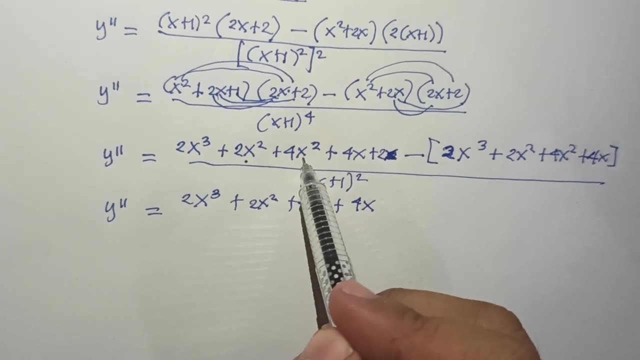 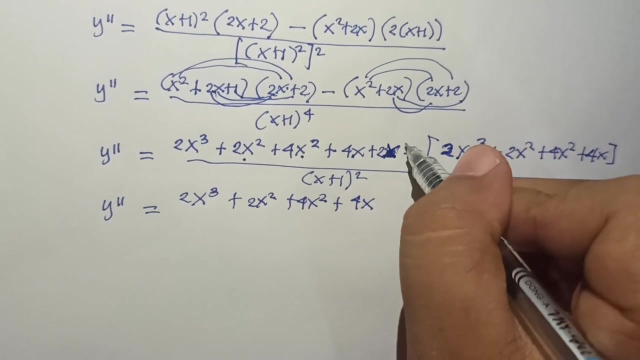 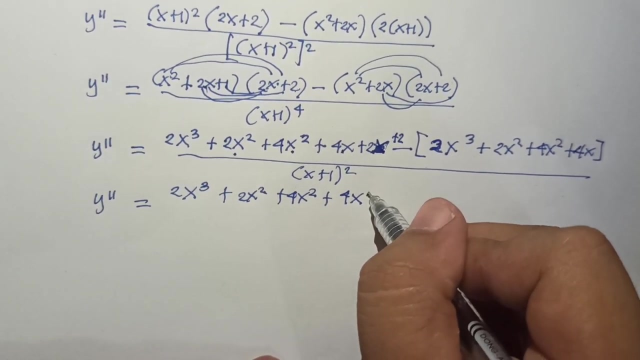 this is 2x cubed plus 2x squared, then 4x squared, then plus 4x squared plus. ah, this is plus 2x and plus 2, so still, we have plus 2 here plus 4x plus. 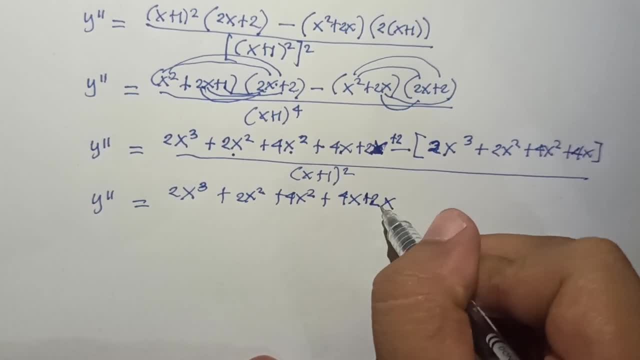 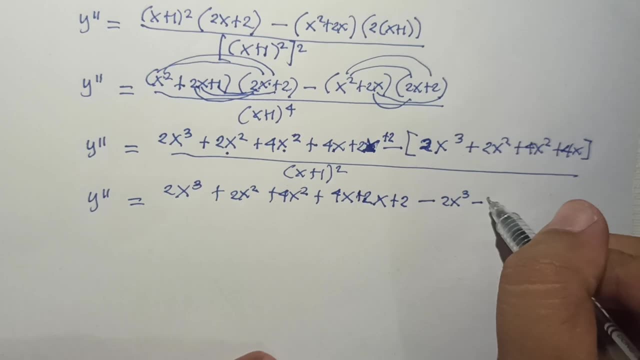 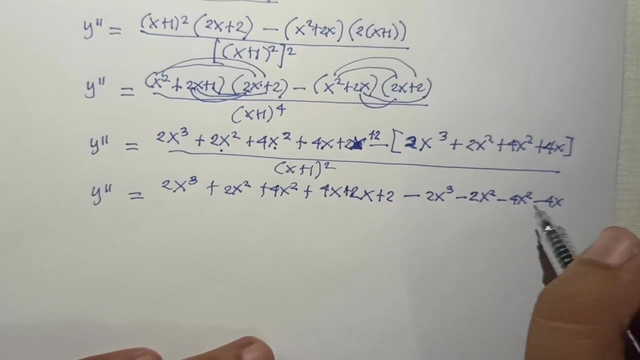 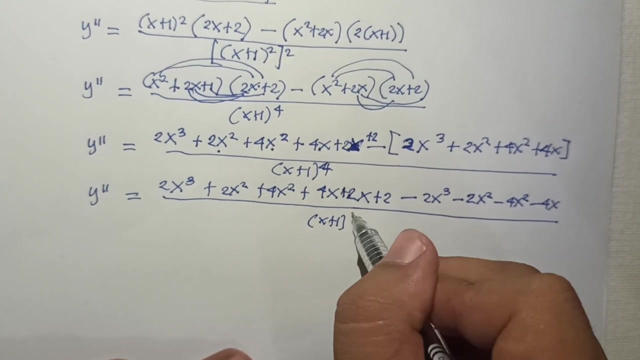 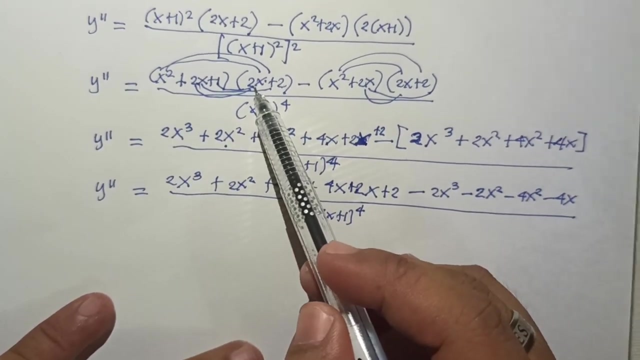 2x plus 2, minus 2x cubed, minus 2x squared minus 4x squared minus 4x. Okay, so over x plus 1, raised to 4, by the way, Again, we're going to go back here. so this is x squared times 2x, that is, 2x cubed then. 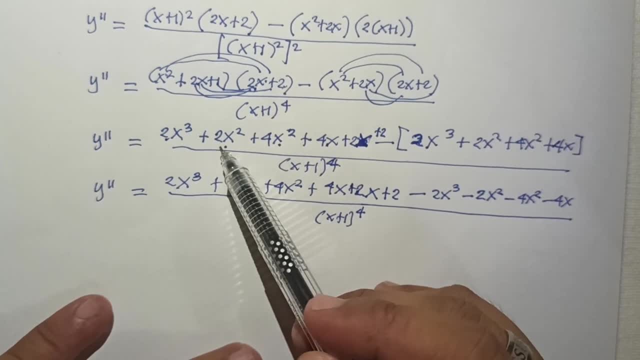 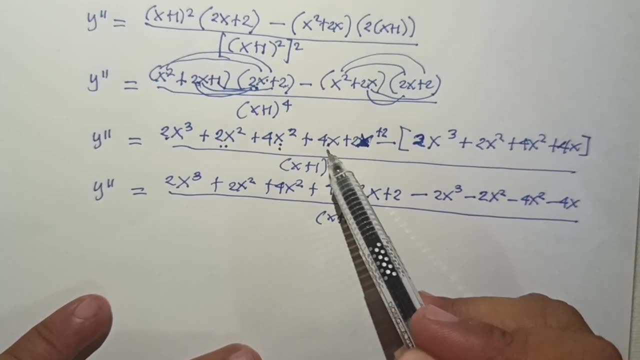 x squared times 2,, that is 2x squared. so 2x times 2x, that is 4x squared. 2x times 2, that is 4x. Then 1 times 2x, that is 4x squared. 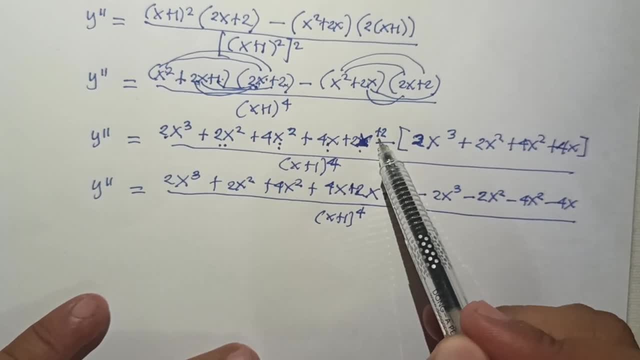 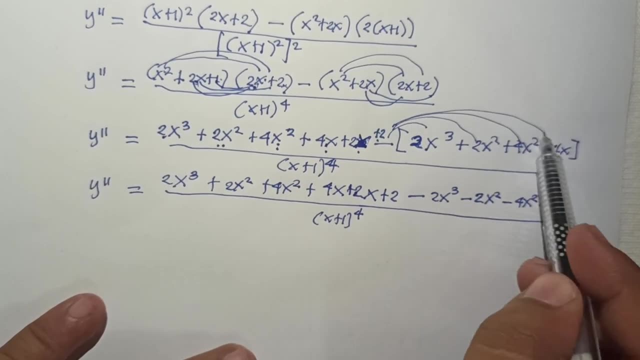 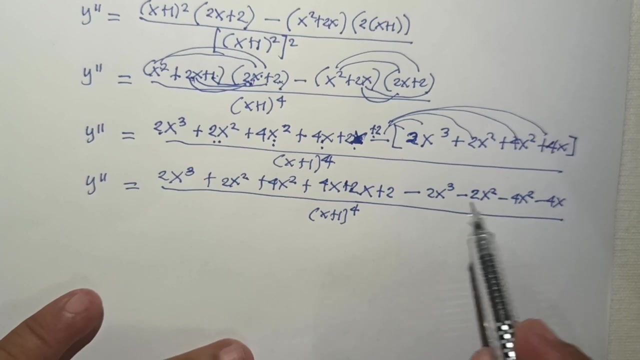 That is 2x and 1 times 2,, that is plus 2,. check And distribute this part, the sign here, so this will come negative: 2x cubed minus 2x squared minus 4x. squared minus 4x. all over: x plus 1 raised to 4.. 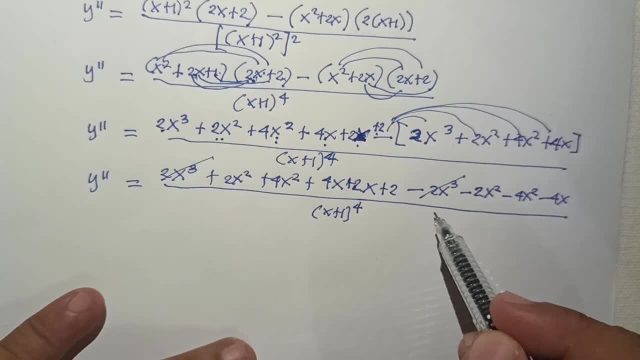 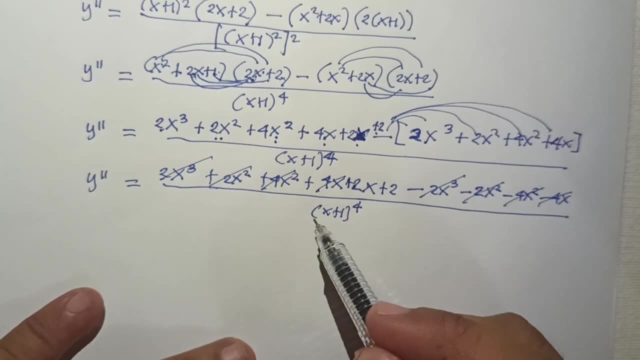 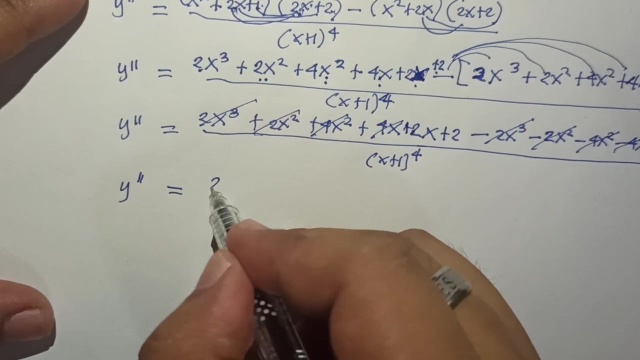 So this time we have to cancel part 2x squared cancel. 4x squared- cancel and 4x also cancel. So the remaining is y double prime is equal to 2x plus 2 over x plus 1 raised to 4.. 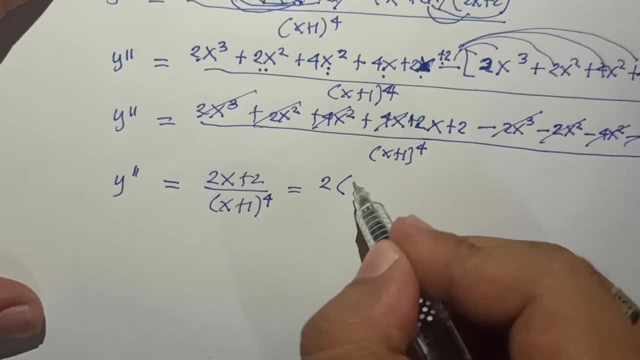 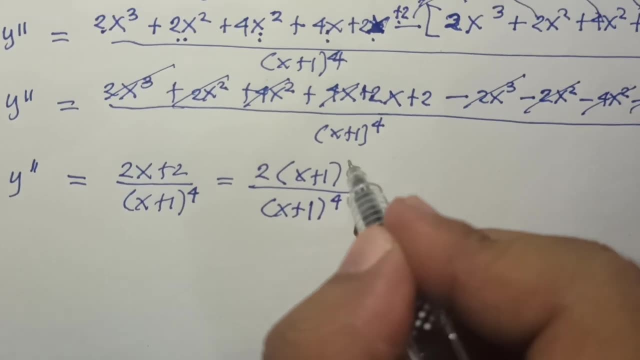 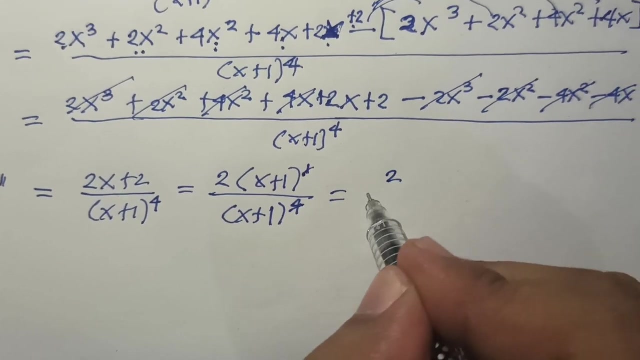 So this is vectorable. so 2x plus 1 over x plus 1 raised to 4.. So this is 1, exponent of 1, so therefore minus. So this is 2 over x plus 1 cubed. 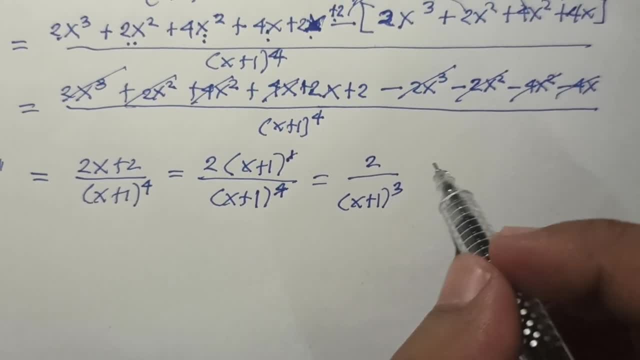 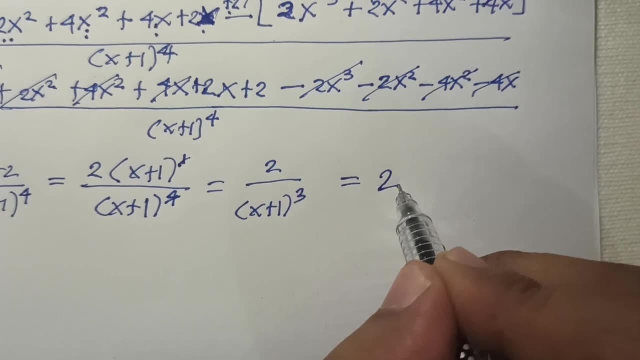 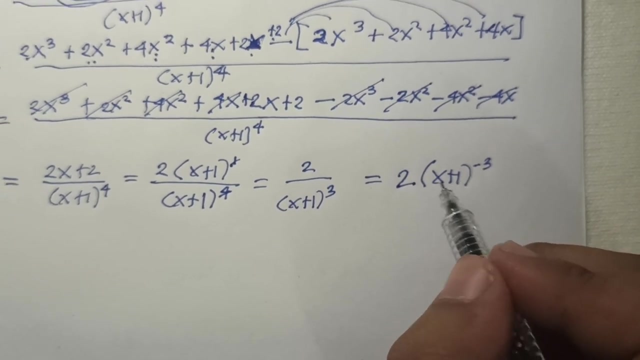 So this is the second derivative. So we could express this in the third derivative for an easy way of differentiating this one. So we have x plus 1 raised to negative 3. So for you to have an easy way of differentiating, we have to put that one into the numerator. 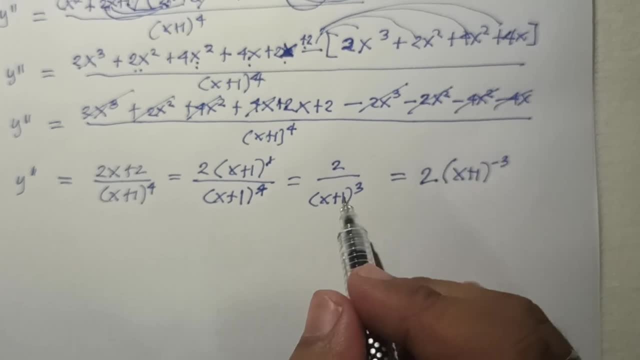 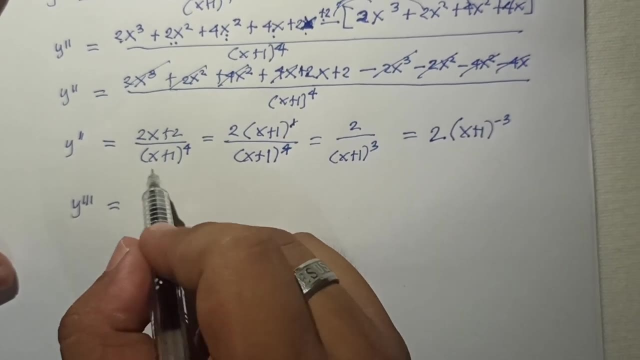 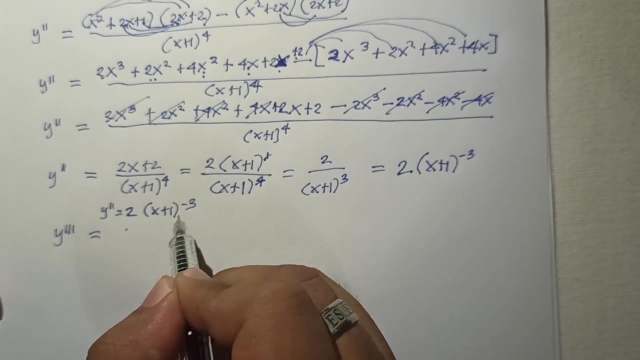 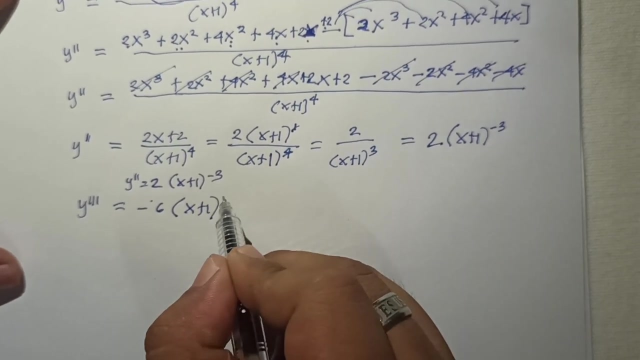 and let it be a negative. So we have x plus 1 raised to negative 3.. So the third derivative- so we have the given, is: y double prime is equal to 2 times x plus 1 raised to negative 3.. So negative 3 times 2, that is negative 6x plus 1 raised to negative 4..